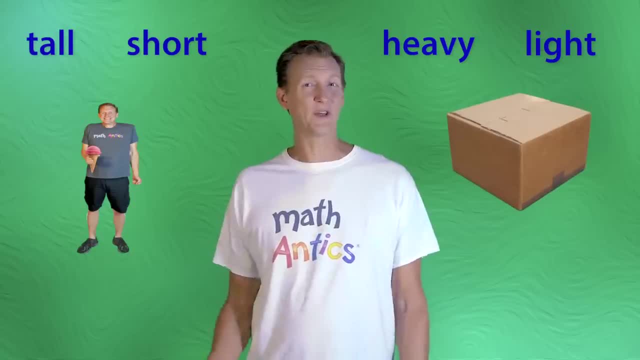 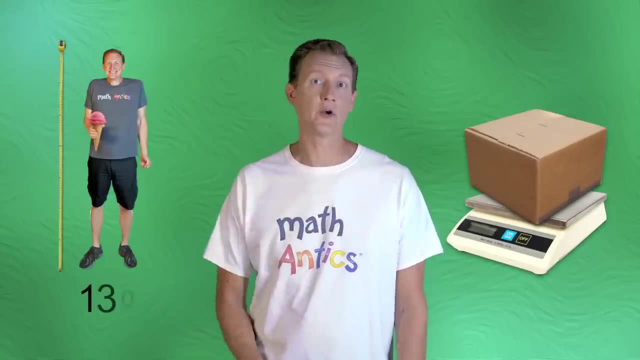 a package is heavy or light, but those are relative terms that don't give us very specific information. Instead, if you were to make actual measurements, you could say that someone's height is 130 centimeters or that a package weighs 5.2 kilograms. Measurements: use an. 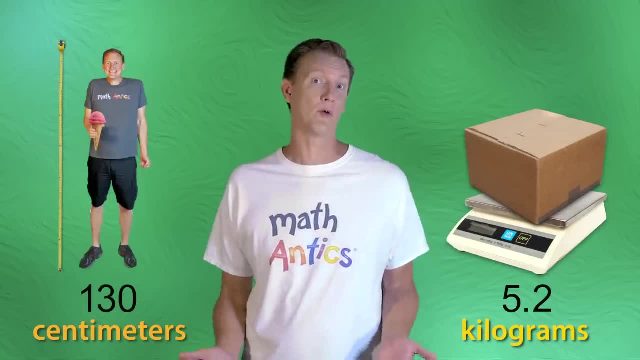 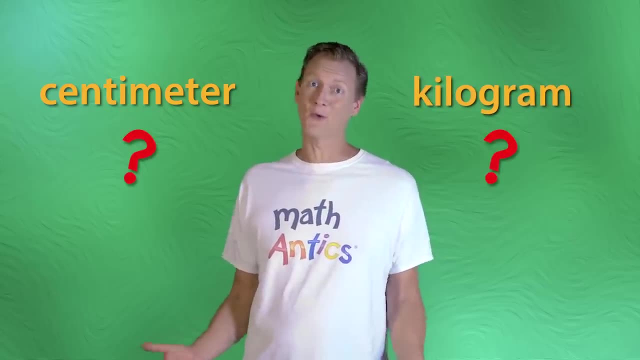 actual number to describe properties like that, so that you can know them more precisely. But there's a catch: Unless you know what a centimeter or a kilogram is, those measurements won't be very helpful. Centimeters and kilograms are examples of what we call units of measurement. 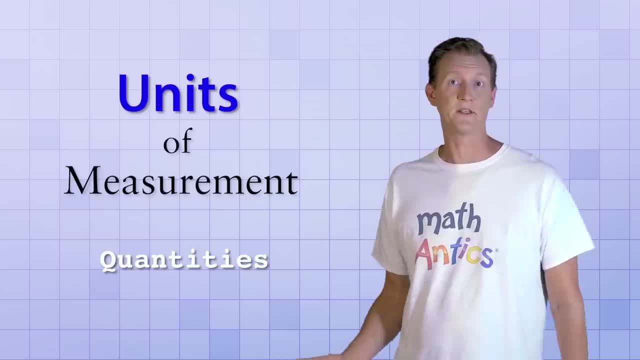 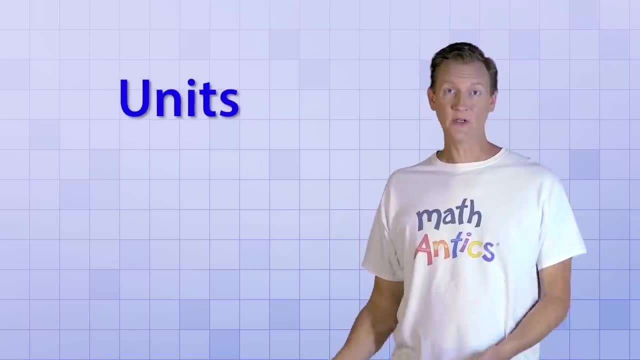 Units of measurement are pre-determined quantities that we use as references, and it's really important to be familiar with common units of measurement so you know what various measurements mean. Units of measurement aren't something fundamental to math like addition and subtraction are. Instead, they're amounts that people 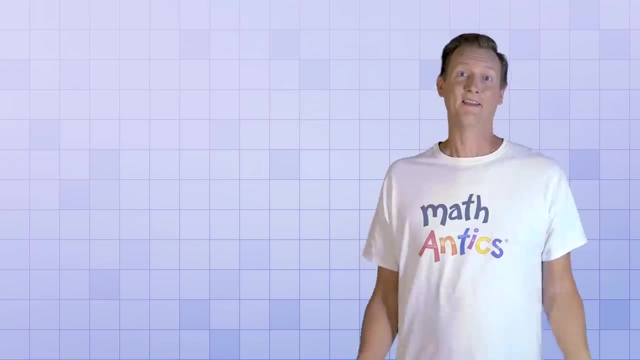 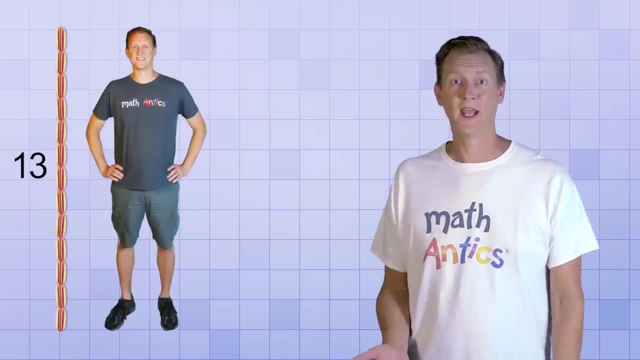 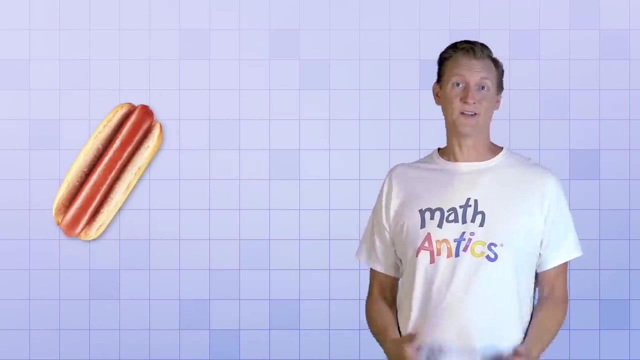 invent and agree on so that we can communicate. In fact, we could agree to use just about anything as a unit of measurement. I could tell you that I'm 13 hot dogs tall and my weight is 3,259 donuts. The problem with those units is that hot dogs and donuts aren't. 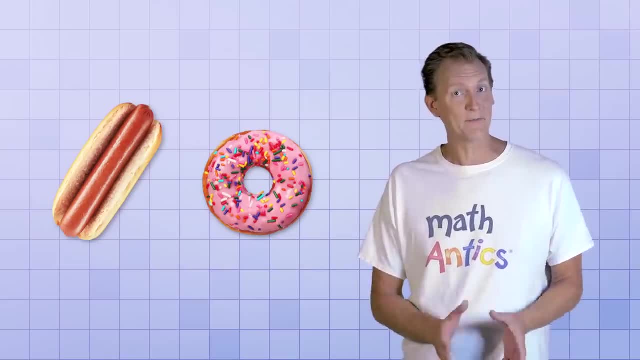 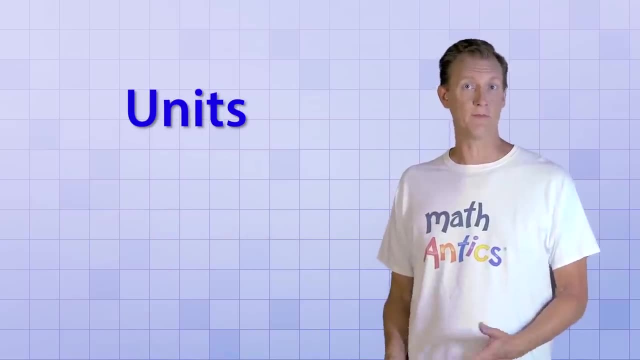 very consistent and unless you and I are using exactly the same hot dogs and donuts to measure, we'll probably come up with different results. To get around this problem, the units that we use in math and science are called units of measurement. The units that we use in math and science are called units of measurement. 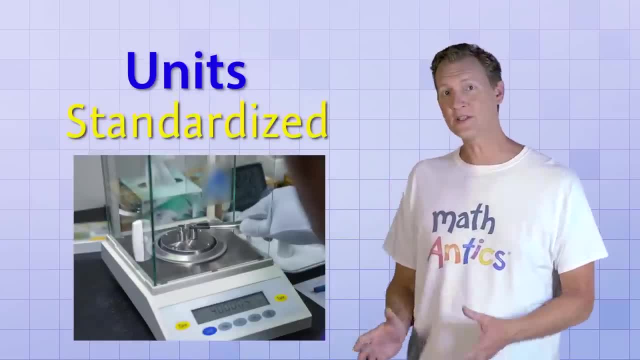 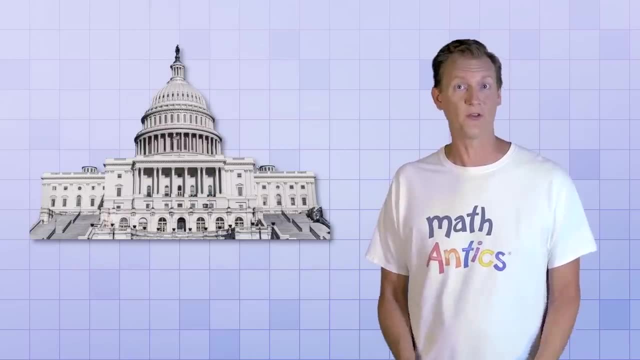 The units that we use in math and science are standardized, which means that they match official standard amounts that can be measured over and over again to give exactly the same result. There's even a government agency called the Bureau of Weights and Measures that defines and maintains those standard amounts. 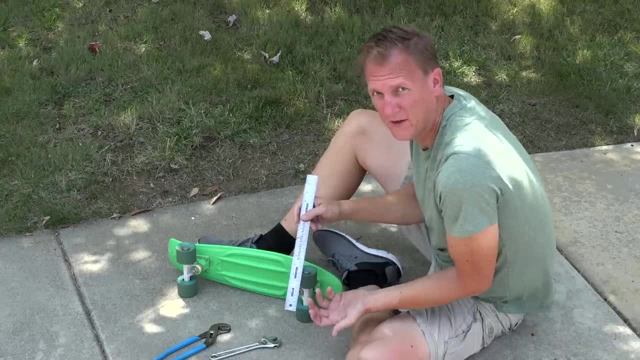 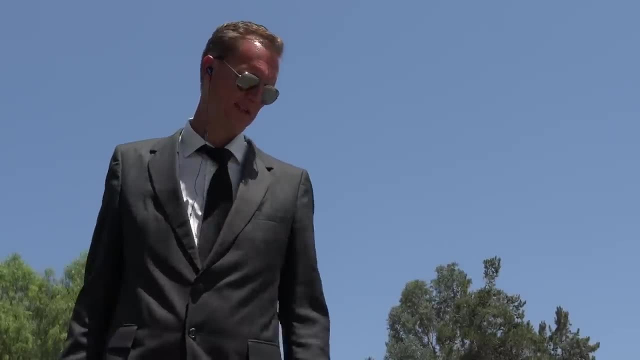 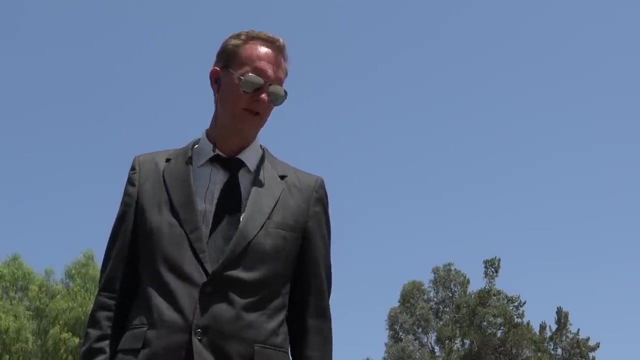 Well, what do we have here? Nothing, Just measuring stuff. Let me see that. Ha, Just as I suspected, This isn't properly calibrated. I just had it checked. Yep, Gonna have to take it into the lab for adjustments. Don't let it happen again. 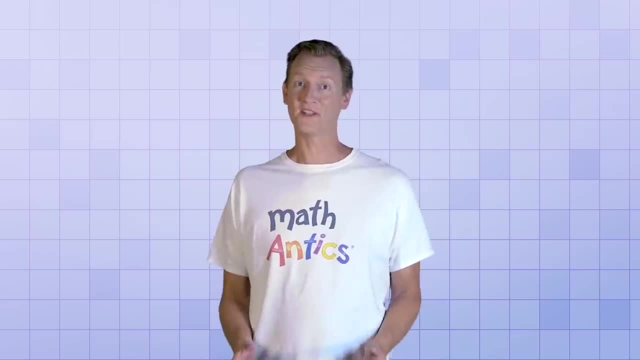 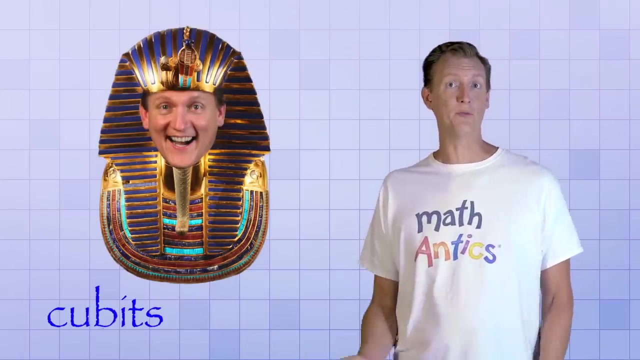 So is there a number? I call to get that back. Of course, getting a bunch of different people to all agree to use the same standards is not always an easy task, and throughout history a variety of different units have come in and out of popularity. For example, the ancient Egyptians used units like cubits and kites. 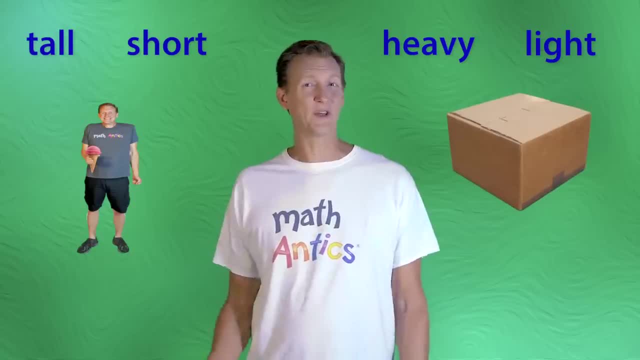 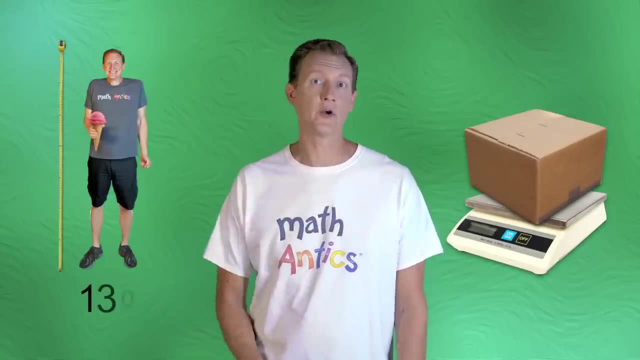 a package is heavy or light, but those are relative terms that don't give us very specific information. Instead, if you were to make actual measurements, you could say that someone's height is 130 centimeters or that a package weighs 5.2 kilograms. Measurements: use an. 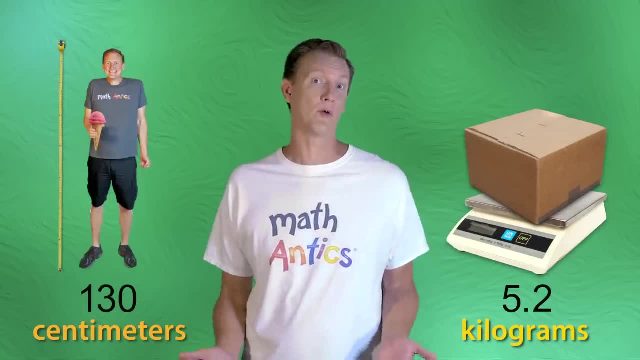 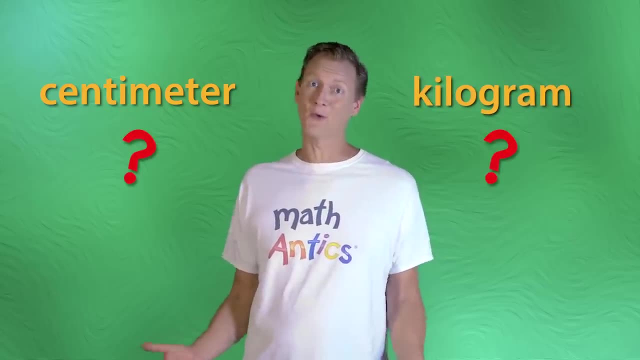 actual number to describe properties like that, so that you can know them more precisely. But there's a catch: Unless you know what a centimeter or a kilogram is, those measurements won't be very helpful. Centimeters and kilograms are examples of what we call units of measurement. 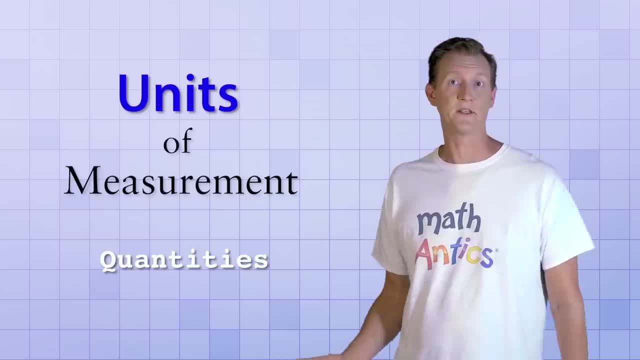 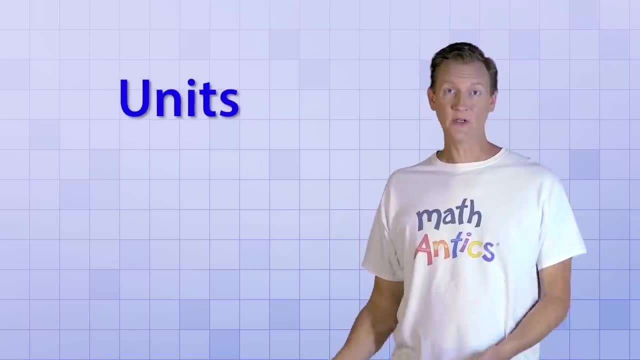 Units of measurement are pre-determined quantities that we use as references, and it's really important to be familiar with common units of measurement so you know what various measurements mean. Units of measurement aren't something fundamental to math like addition and subtraction are. Instead, they're amounts that people 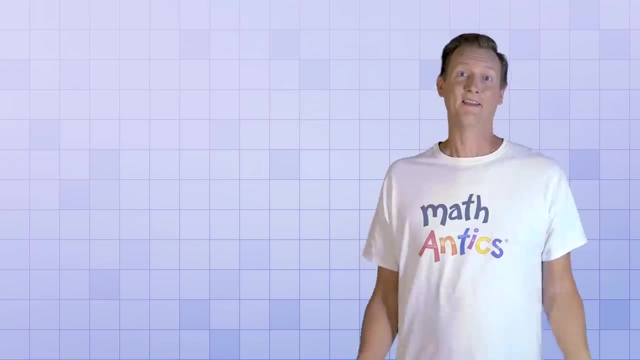 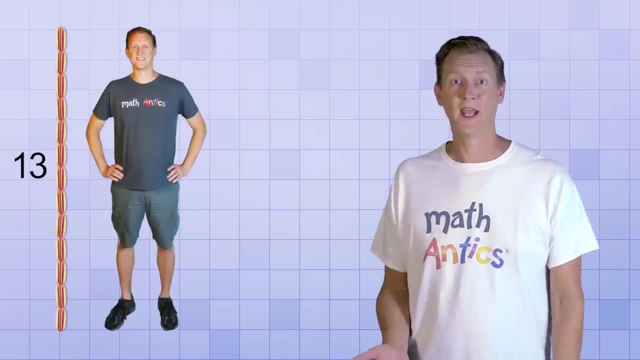 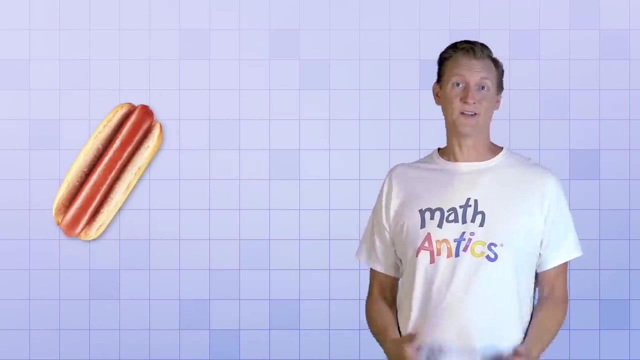 invent and agree on so that we can communicate. In fact, we could agree to use just about anything as a unit of measurement. I could tell you that I'm 13 hot dogs tall and my weight is 3,259 donuts. The problem with those units is that hot dogs and donuts aren't. 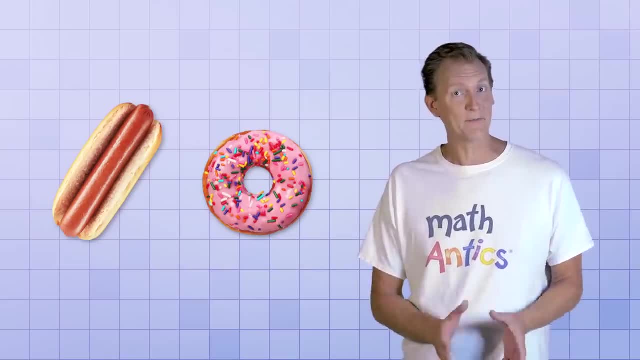 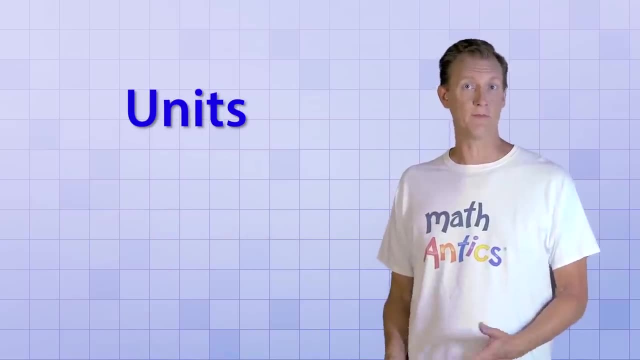 very consistent and unless you and I are using exactly the same hot dogs and donuts to measure, we'll probably come up with different results. To get around this problem, the units that we use in math and science are called units of measurement. The units that we use in math and science are called units of measurement. 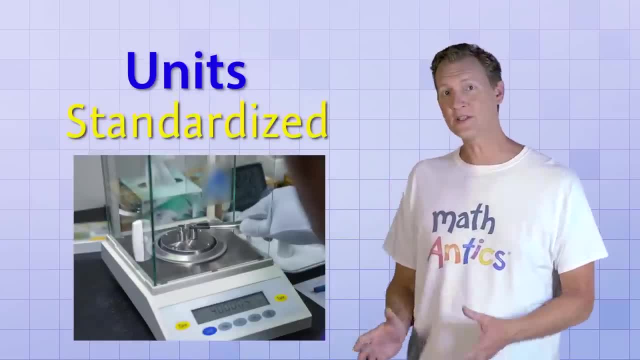 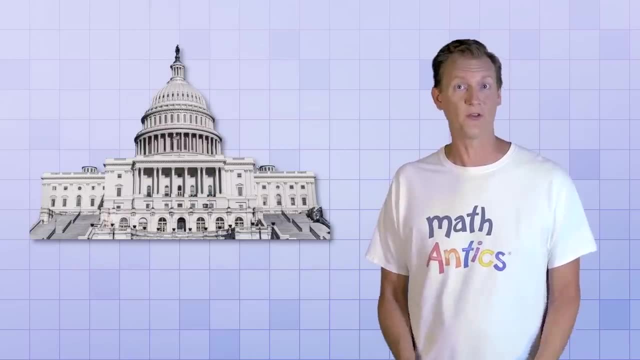 The units that we use in math and science are standardized, which means that they match official standard amounts that can be measured over and over again to give exactly the same result. There's even a government agency called the Bureau of Weights and Measures that defines and maintains those standard amounts. 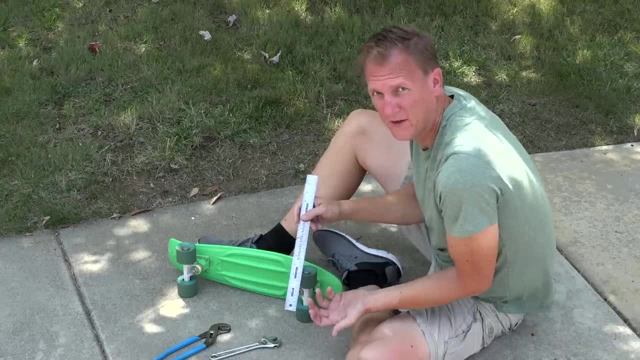 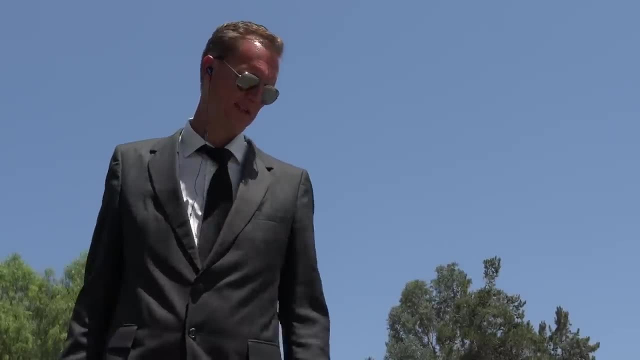 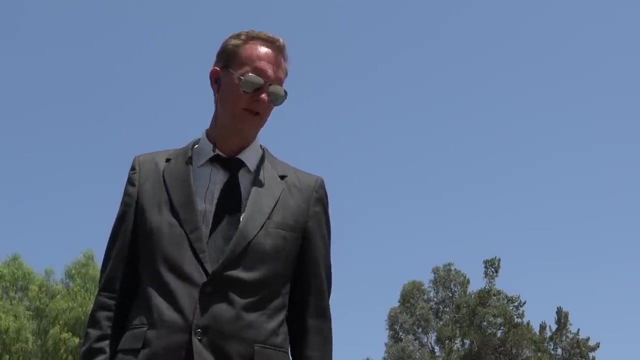 Well, what do we have here? Nothing, Just measuring stuff. Let me see that. Ha, Just as I suspected, This isn't properly calibrated. I just had it checked. Yep, Gonna have to take it into the lab for adjustments. Don't let it happen again. 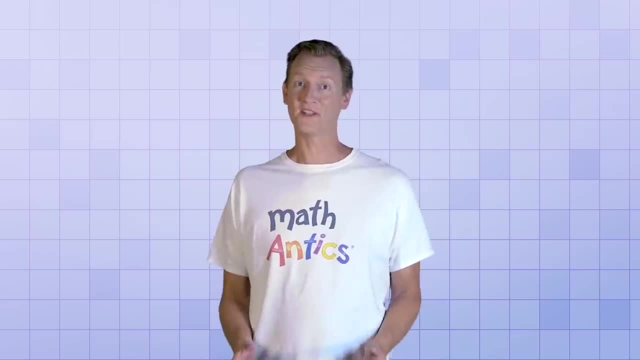 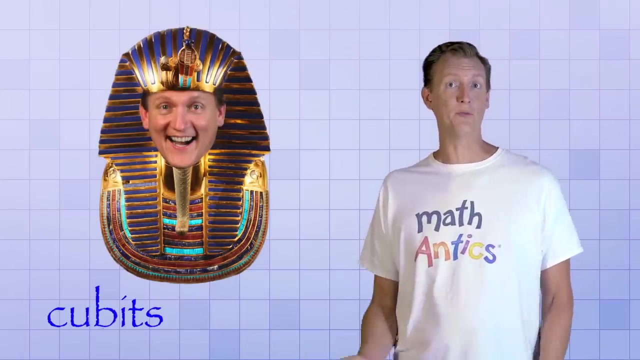 So is there a number? I call to get that back. Of course, getting a bunch of different people to all agree to use the same standards is not always an easy task, and throughout history a variety of different units have come in and out of popularity. For example, the ancient Egyptians used units like cubits and kites. 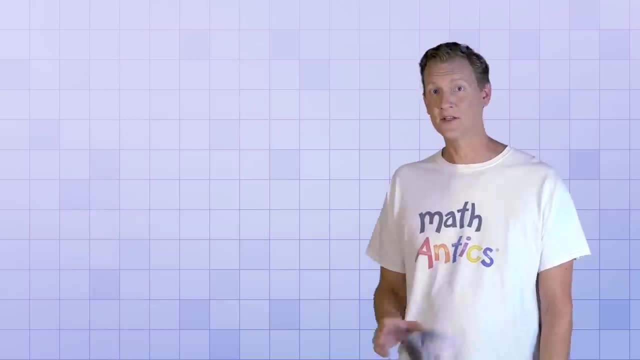 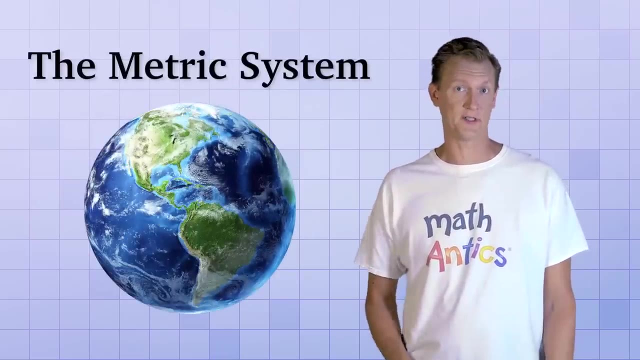 which aren't so popular today. In modern times, there are still a lot of different units that are used in different countries, But the most popular system of units used around the world is called the metric system. Well, its official name is the International System of Units. 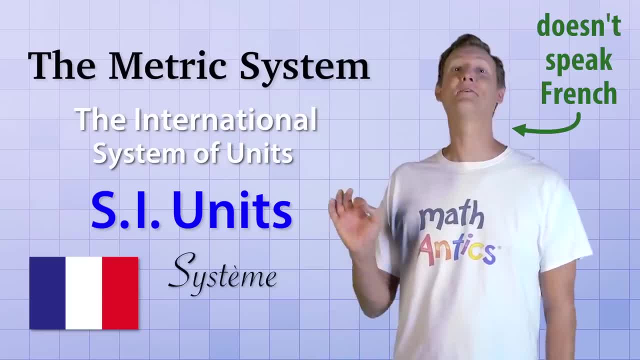 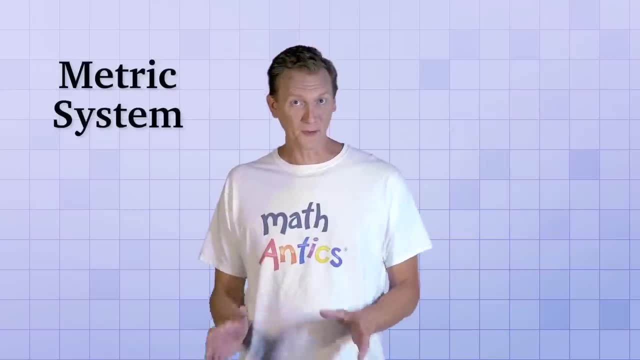 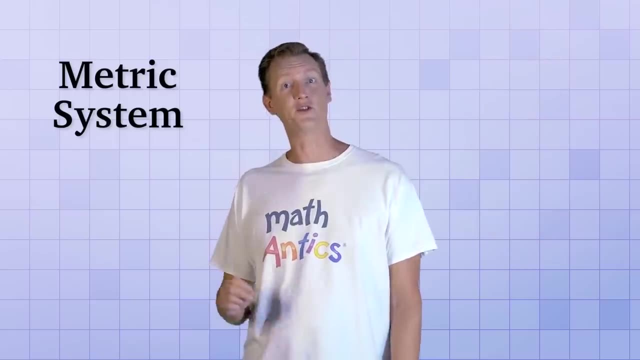 or SI Units for short, which stands for the French Système International, But the term metric system is still often used to refer to this system. The metric system is a really great idea because it makes the math involved with certain measurements and unit conversion much easier to do. That's because, just like our base 10 number system, 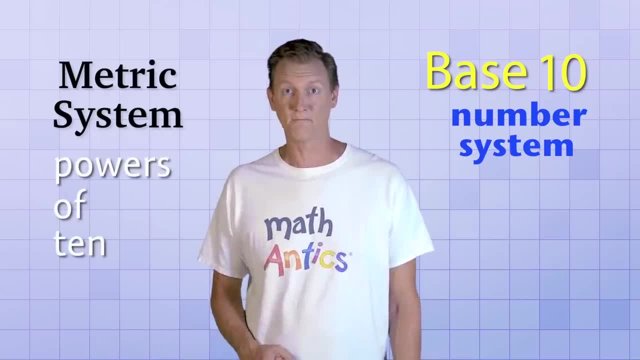 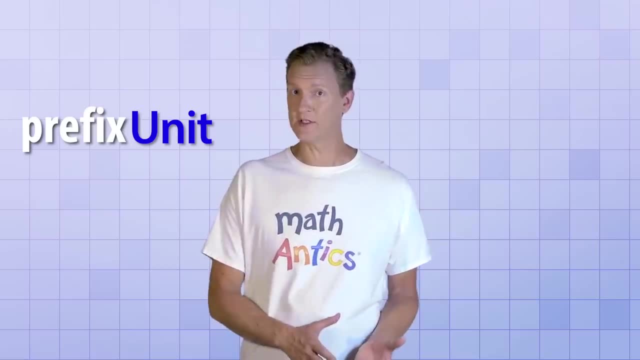 most units in the metric system take advantage of powers of 10.. The idea behind the metric system is to start with a base unit and then use standard prefixes to make other units that are bigger or smaller than that base unit by powers of 10.. 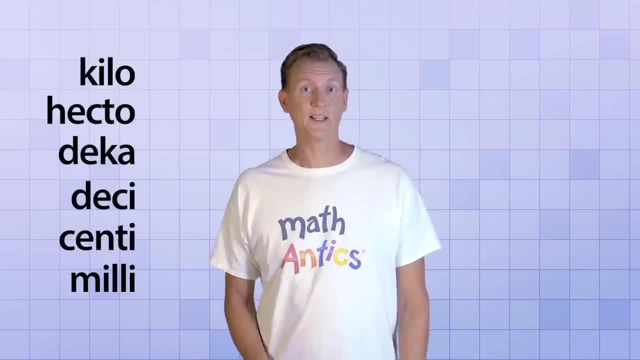 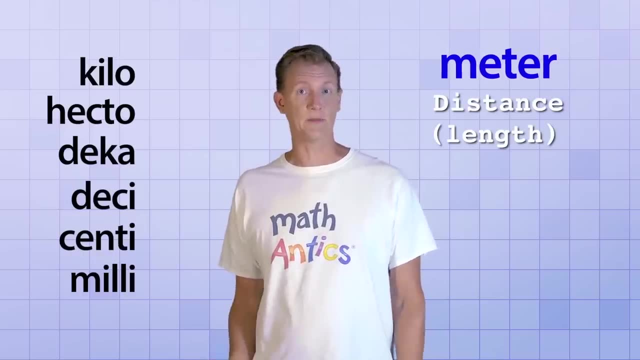 Here's a list of some of those prefixes To see how they work. let's consider a key unit in the metric system called a meter. A meter is a basic unit of distance or length, and it happens to be about this long. 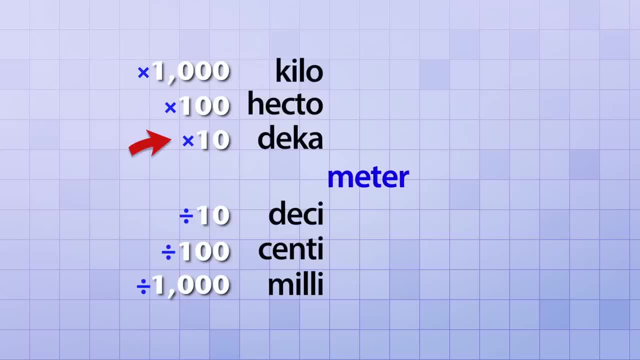 As you can see from our prefixes, the unit that's 10 meters long is called a meter. The unit that's 10 times bigger than a meter is called a decameter. The unit that's 100 times bigger than a meter is called a hectameter. 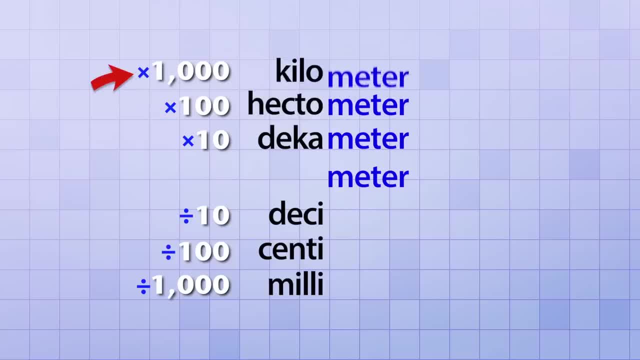 And the unit that's 1000 times bigger than a meter is called a kilometer or a kilometer. But this system also has prefixes to define units that are smaller than a meter. The unit that's 10 times smaller or one-tenth of a meter is called a decimeter. 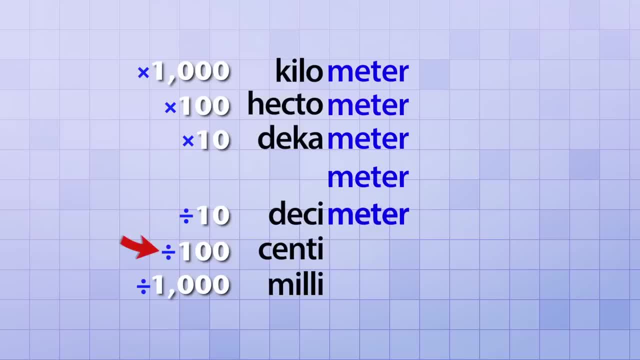 The unit that's 100 times smaller or one-hundredth of a meter is called a centimeter, And the unit that's 1000 times smaller or one-thousandth of a meter is called a centimeter. Get the idea. 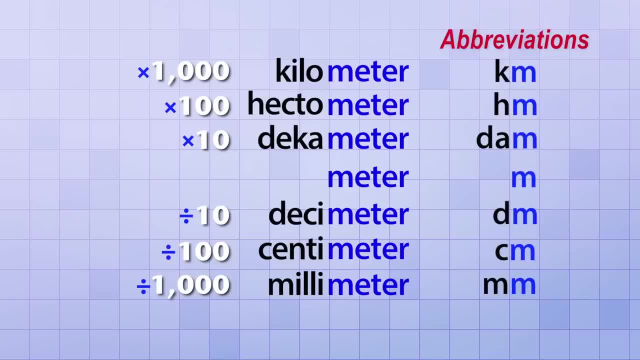 There are also abbreviations for each of these units to make writing them down a lot more convenient. A meter is just abbreviated as M, And then you put other letters in front of that for the other units. For example, a kilometer is abbreviated KM, while a centimeter is abbreviated CM. 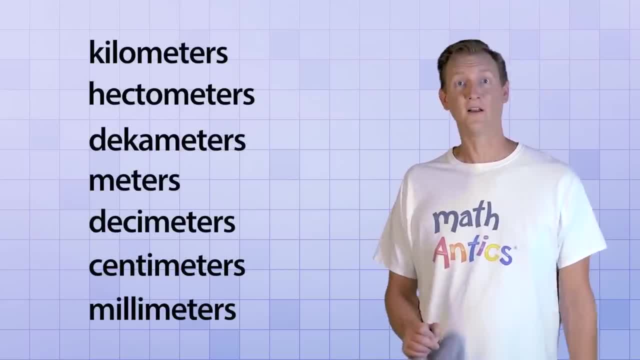 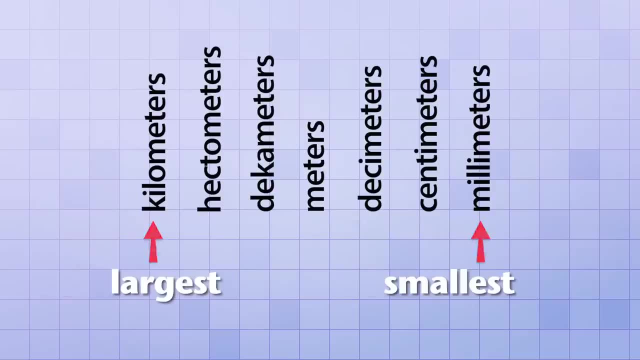 So why does the metric system make working with units easier? Well, notice the pattern we get if we put these units in order, with the largest unit on the left and the smallest unit on the right. Each unit is 10 times bigger than the unit immediately on its right. 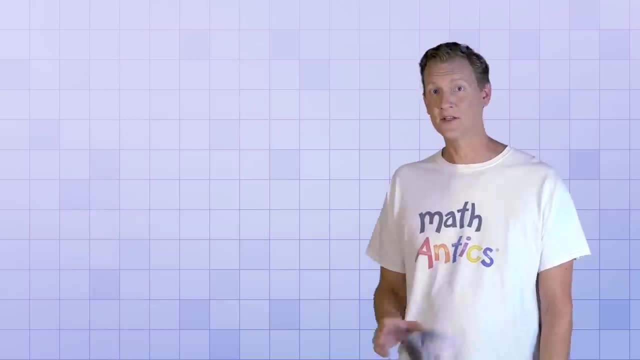 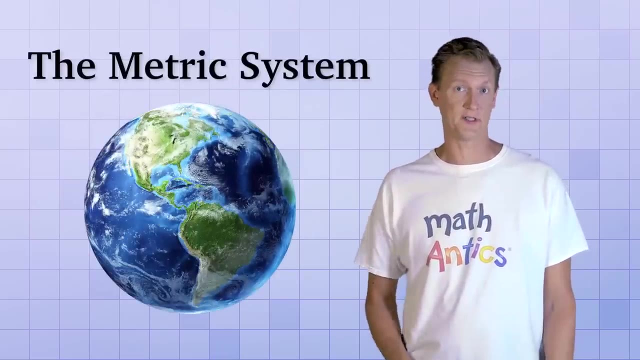 which aren't so popular today. In modern times, there are still a lot of different units that are used in different countries, But the most popular system of units used around the world is called the metric system. Well, its official name is the International System of Units. 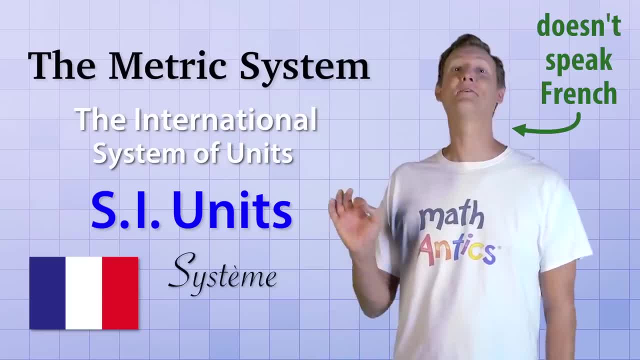 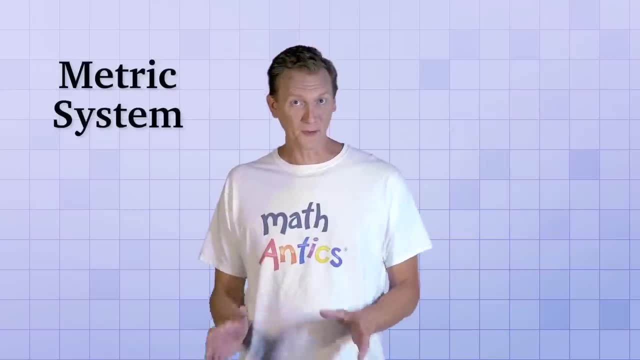 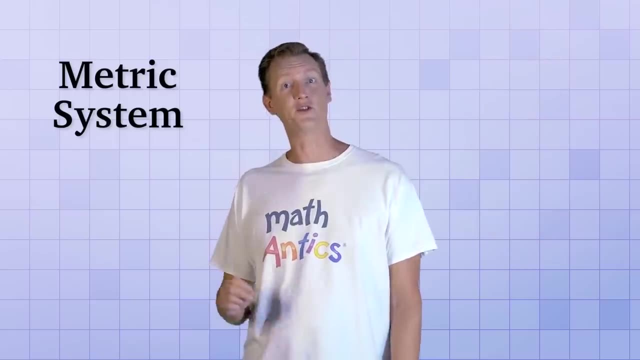 or SI Units for short, which stands for the French Système International, But the term metric system is still often used to refer to this system. The metric system is a really great idea because it makes the math involved with certain measurements and unit conversion much easier to do. That's because, just like our base 10 number system, 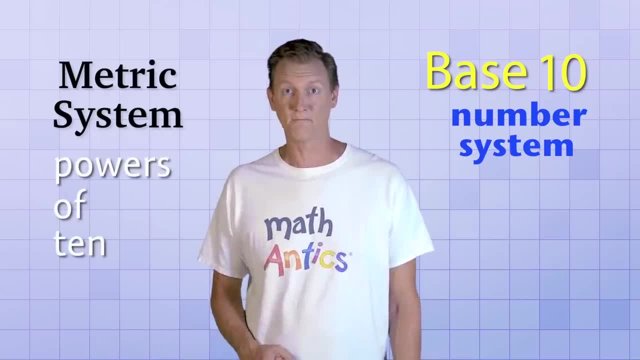 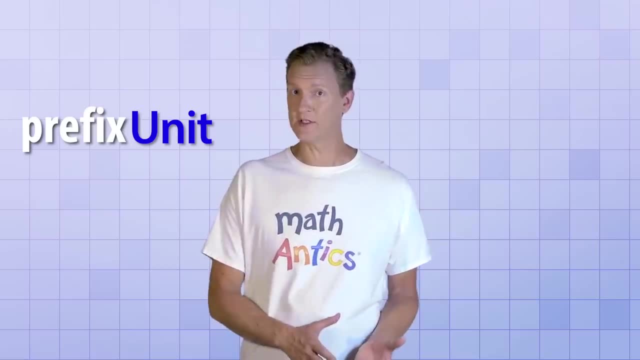 most units in the metric system take advantage of powers of 10.. The idea behind the metric system is to start with a base unit and then use standard prefixes to make other units that are bigger or smaller than that base unit by powers of 10.. 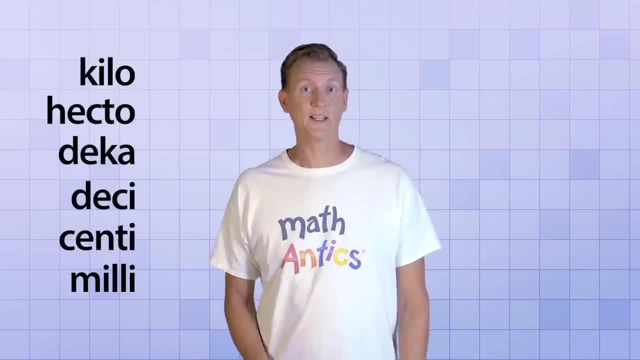 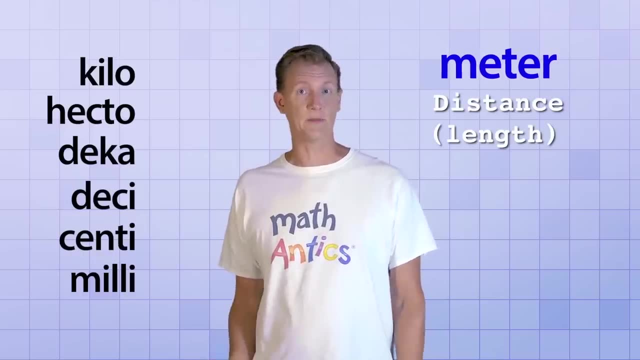 Here's a list of some of those prefixes To see how they work. let's consider a key unit in the metric system called a meter. A meter is a basic unit of distance or length, and it happens to be about this long. As you can see from our prefixes, the unit that's 10 meters long is the unit that's 10 meters long. As you can see from our prefixes, the unit that's 10 meters long is the unit that's 10 meters long. 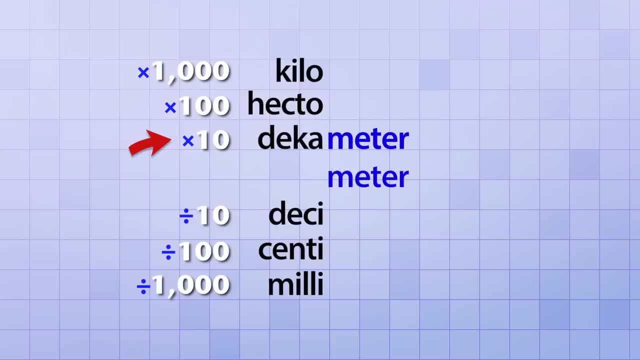 The unit that's 10 times bigger than a meter is called a decameter, The unit that's 100 times bigger than a meter is called a hectameter, And the unit that's 1000 times bigger than a meter is called a kilometer or a kilometer. 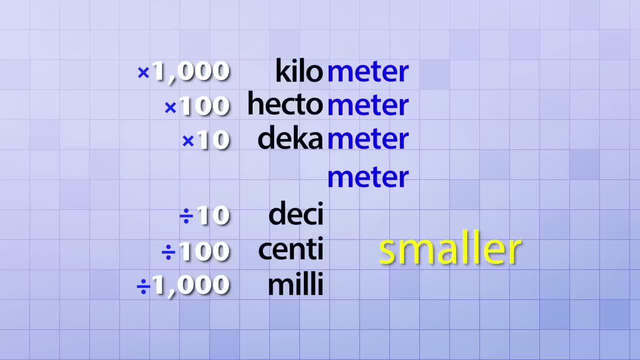 But this system also has prefixes to define units that are smaller than a meter. The unit that's 10 times smaller or one-tenth of a meter is called a decimeter. The unit that's 100 times smaller or one-hundredth of a meter is called a centimeter. And the unit that's 1000 times smaller or one-thousandth of a meter is called a centimeter, And the unit that's 100 times smaller or one-hundredth of a meter is called a centimeter. 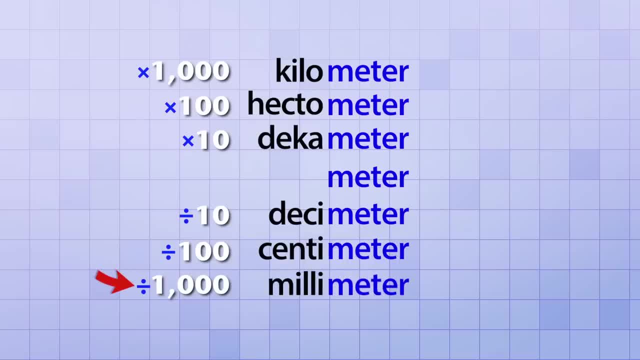 And the unit that's 1000 times smaller, or one-thousandth of a meter, is called a centimeter. a meter is called a millimeter- Get the idea. There are also abbreviations for each of these units to make writing them down a lot more convenient. 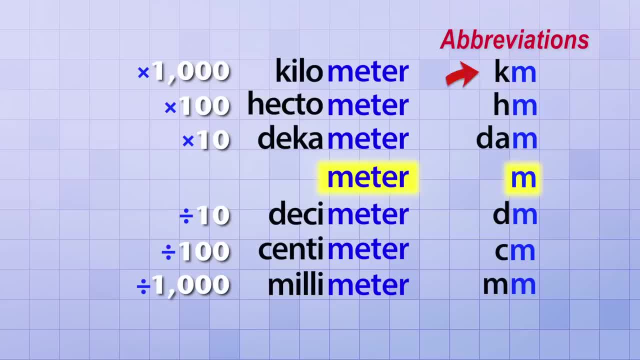 A meter is just abbreviated as M, and then you put other letters in front of that for the other units. For example, a kilometer is abbreviated KM, while a centimeter is abbreviated CM. So why does the metric system make working with units easier? 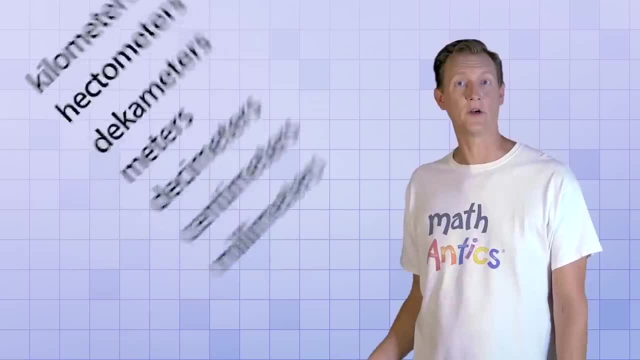 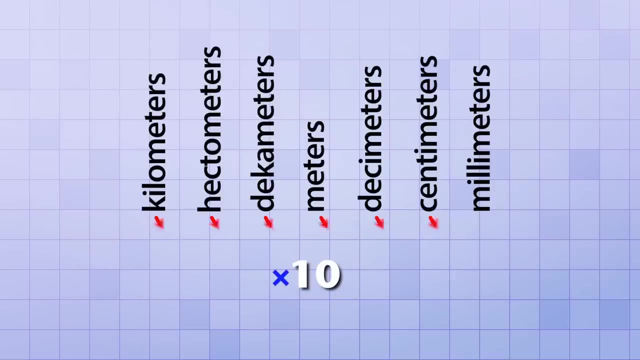 Well notice the pattern we get if we put these units in order, with the largest unit on the left and the smallest unit on the right. Each unit is 10 times bigger than the unit immediately on its right and 10 times smaller than the unit immediately on its left. 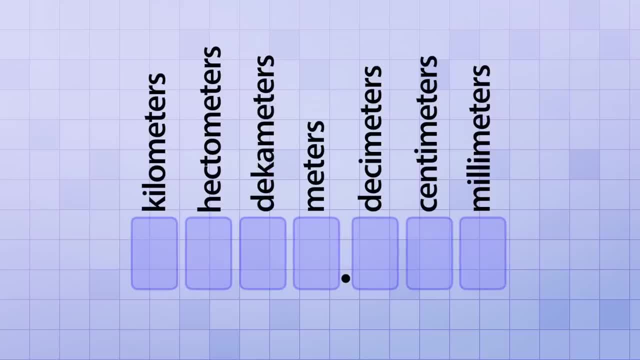 That's exactly the same pattern that the number places use in our decimal number system. This diagram can give you an idea of how the units relate to each other. For example, 1 kilometer is the same as 1000 meters and 1 millimeter is the same as .0001.. 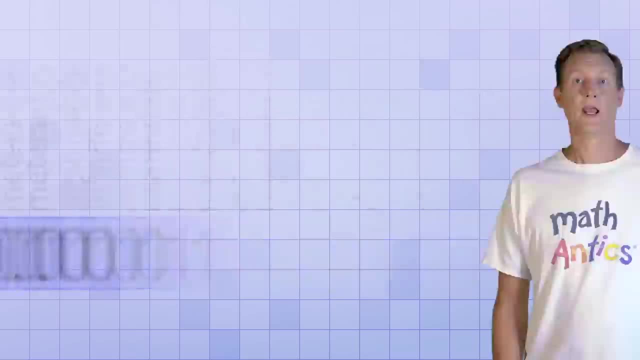 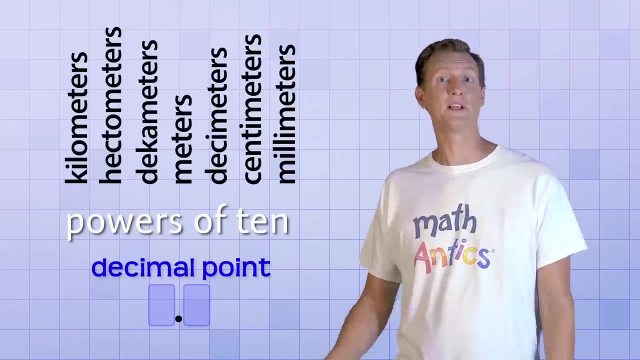 And because all these different units of length are based on powers of 10, you can convert between them just by shifting the decimal point one place at a time, which is equivalent to either multiplying or dividing by 10, depending on which direction you shift. 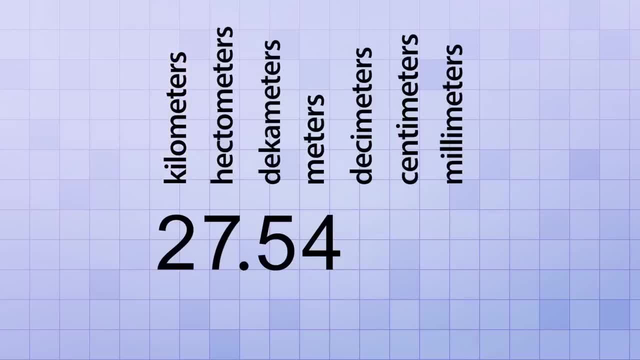 2.754 kilometers is the same as 27.54 hectometers, which is the same as 275.4 decameters, which is the same as 2755.5 hectometers, which is the same as 2755.5 hectometers. 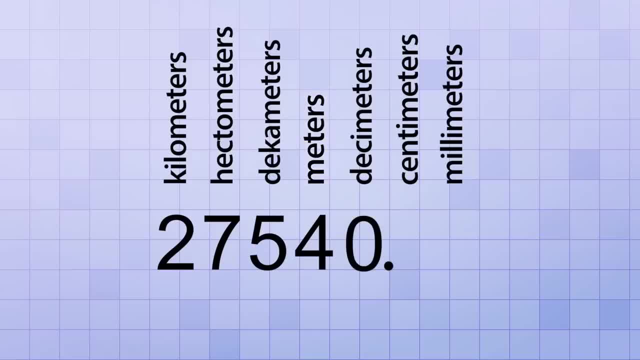 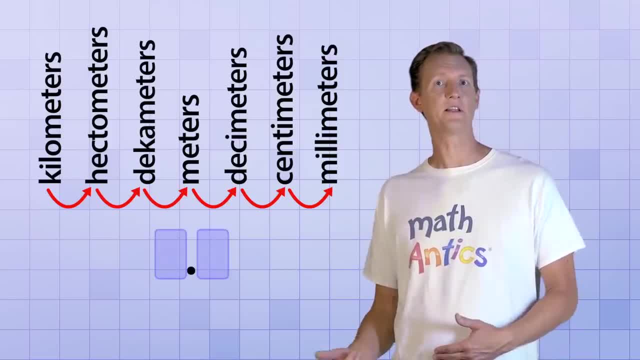 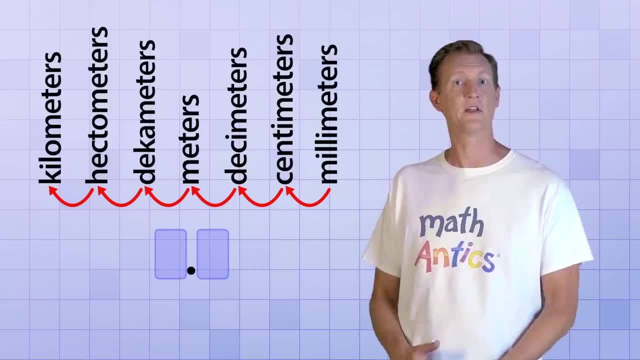 You can convert to the next smaller metric unit by shifting the decimal point to the right, which is equivalent to multiplying by 10.. And you can convert to the next bigger metric unit by shifting the decimal point to the left, which is equivalent to dividing by 10.. 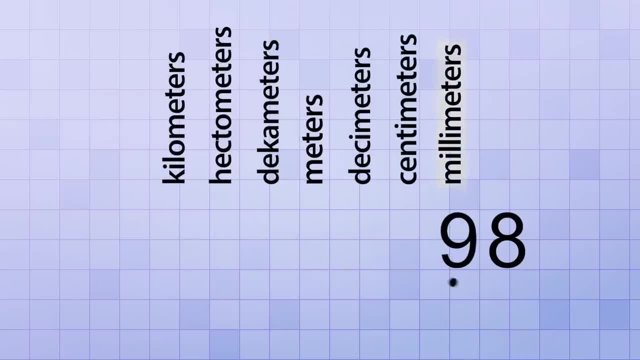 For example, 9.8 millimeters is the same as 0.98 centimeters, which is the same as 0.002 centimeters, which is equivalent to 0.098 decameters, which is the same as 0.0098 meters, and so on. 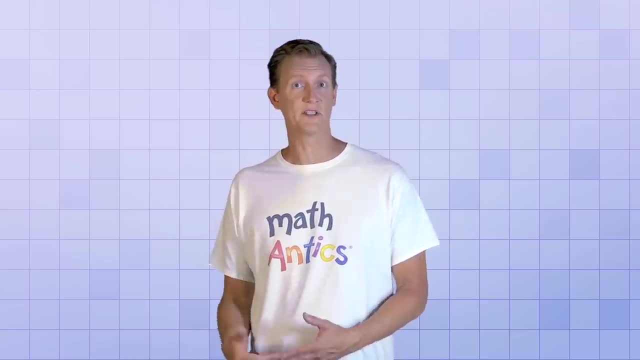 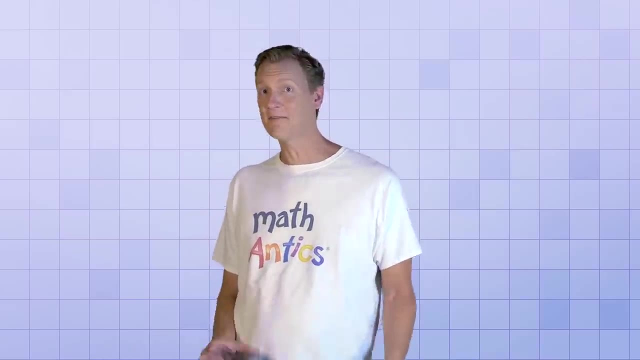 So you can see why the metric system is so useful. It was designed with our number system in mind, which makes it easy to work with Ugh, and even though the metric system defines a lot of different units with all these prefixes, not all are equally popular. 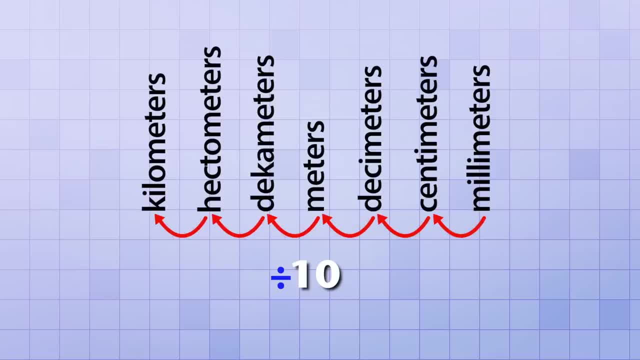 and 10 times smaller than the unit immediately on its left. That's exactly the same pattern that the number places use in our decimal number system. This diagram can give you an idea of how the units relate to each other. For example, 1 kilometer is the same as 1000 meters. 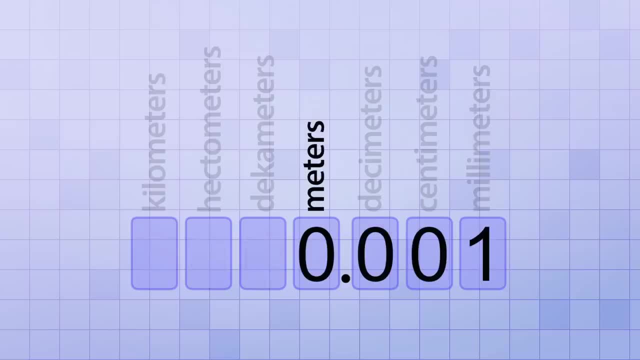 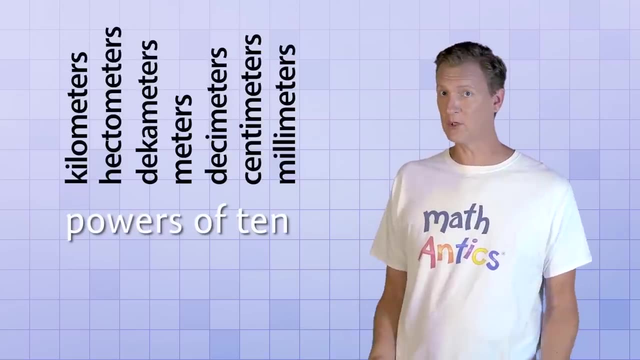 and 1 millimeter is the same as .001 meters, or one-one-thousandth of a meter, And because all these different units of length are based on powers of 10, you can convert between them just by shifting the decimal point one place at a time. 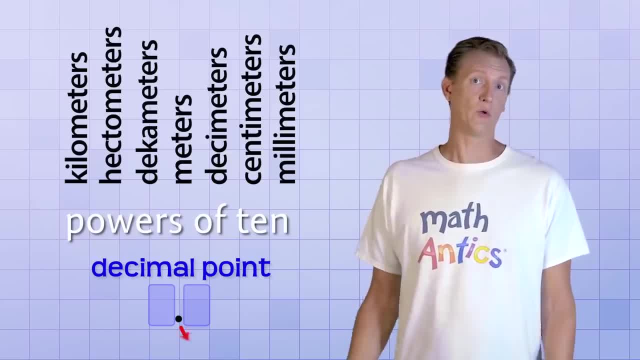 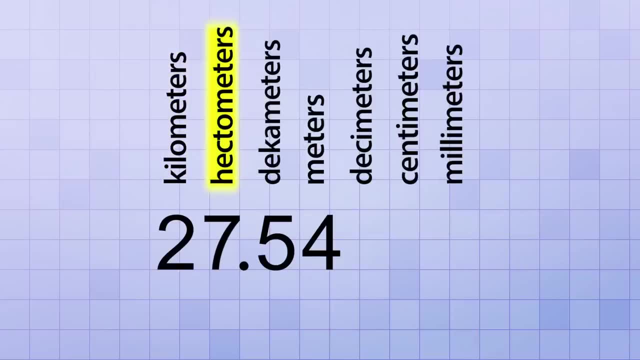 which is equivalent to either multiplying or dividing by 10,, depending on which direction you shift. 2.754 kilometers is the same as 27.54 hectometers, which is the same as 275.4 decameters, which is the same as 2,754 meters. 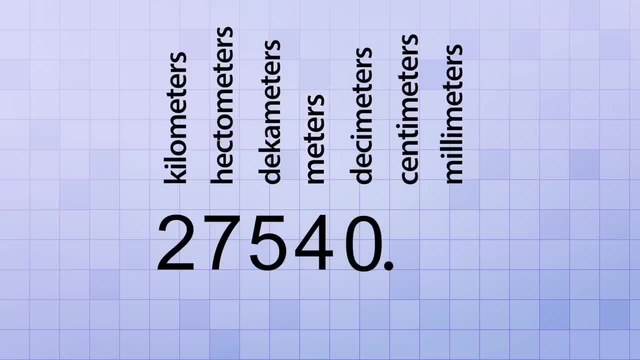 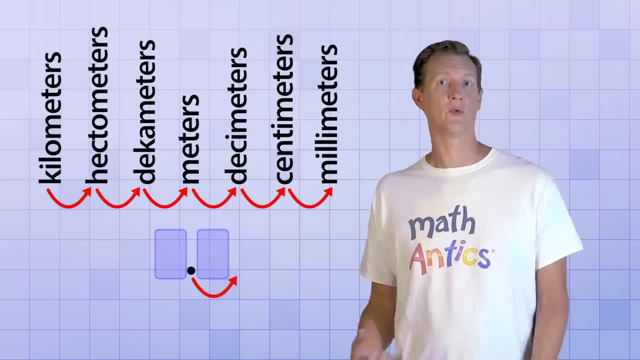 which is the same as 27,000 meters, which is the same as 540 decameters, and so on. You can convert to the next smaller metric unit by shifting the decimal point to the right, which is equivalent to multiplying by 10.. 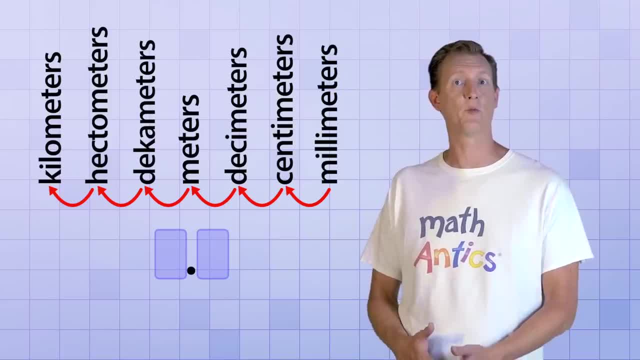 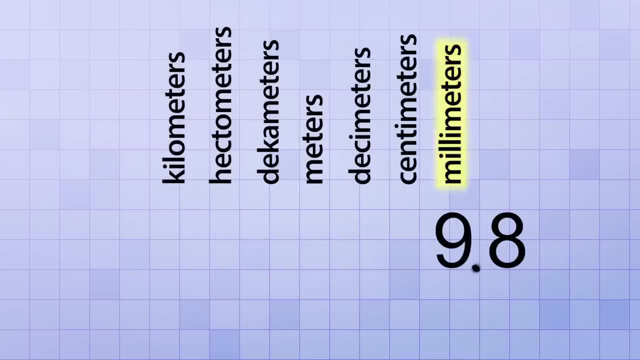 And you can convert to the next bigger metric unit by shifting the decimal point to the left, which is equivalent to dividing by 10.. For example, 9.8 millimeters is the same as 0.98 centimeters, which is the same as 0.098 decameters. 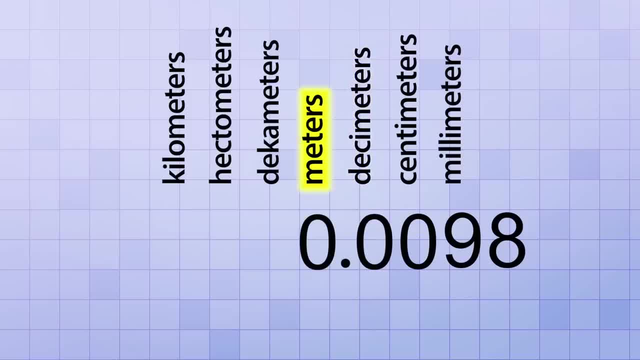 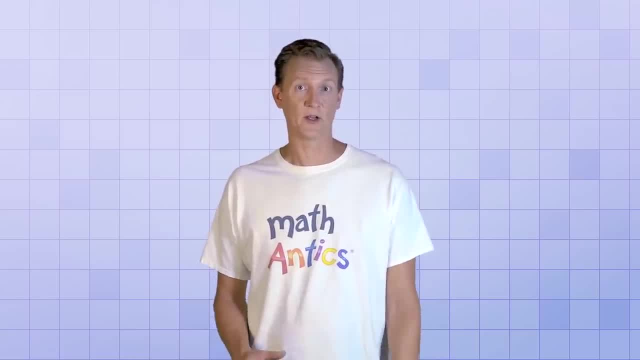 which is the same as 0.001 meters, which is the same as 0.0098 meters, and so on. So you can see why the metric system is so useful. It was designed with our number system in mind, which makes it easy to work with. 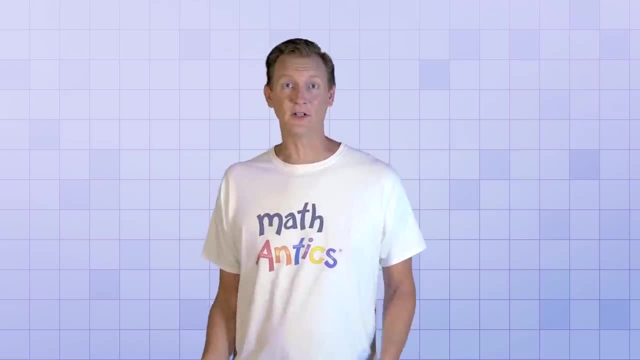 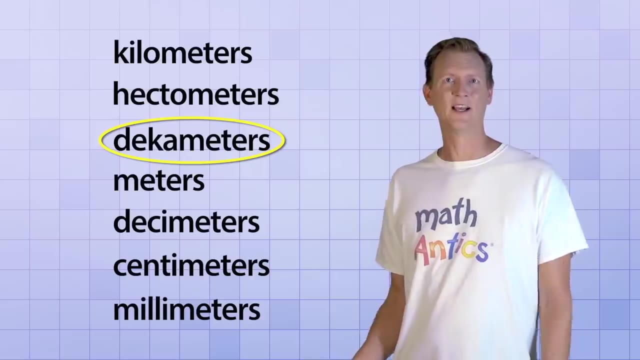 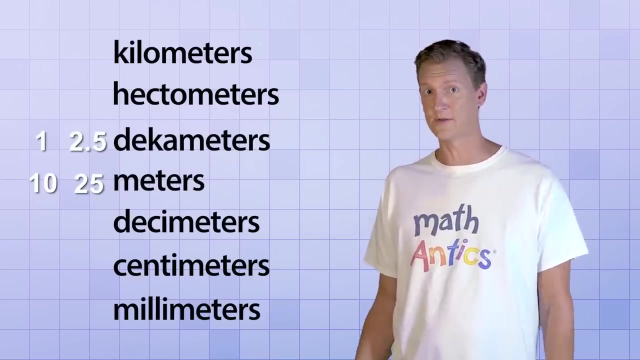 Oh, and even though the metric system defines a lot of different units with all these prefixes, not all are equally popular. For example, it's not very common for people to use decameters. They'll usually just say 10 meters or 25 meters, instead of saying 1 decameter or 2.5 decameters. 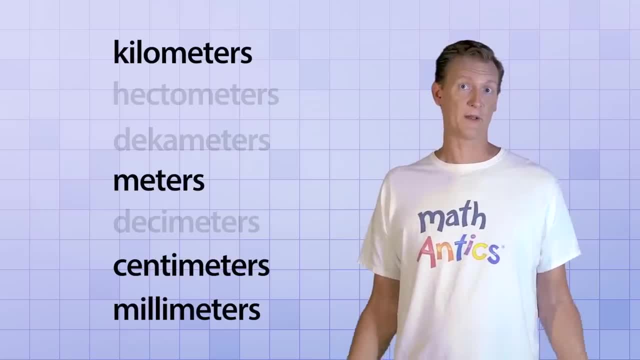 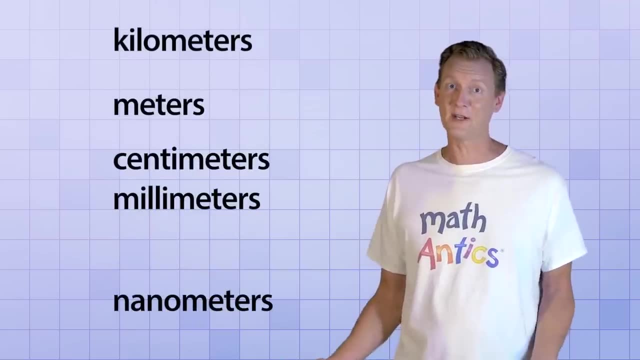 In fact, there's really just 4 metric units of length that are frequently used, And they are the millimeter, the centimeter, the meter and the kilometer. Oh, and, of course, nanometers are commonly used when referring to teeny, tiny stuff like microbes or computer chips. 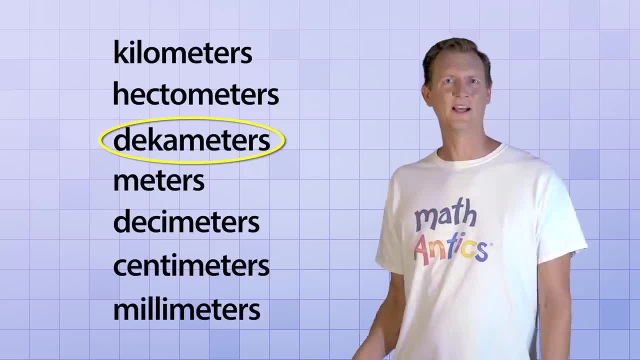 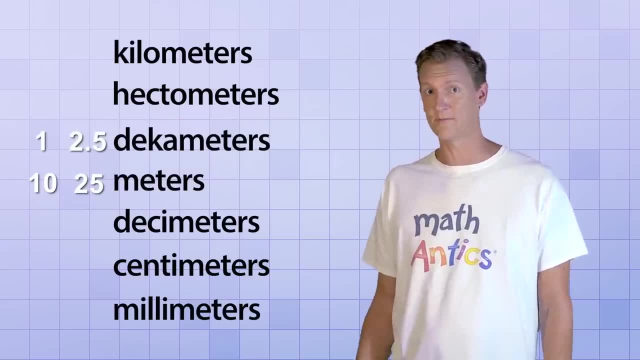 For example, it's not very common for people to use decameters. They'll usually just say 10 meters or 25 meters instead of saying 1 decameter. In fact, there's really just 4 metric units of length that are frequently used. 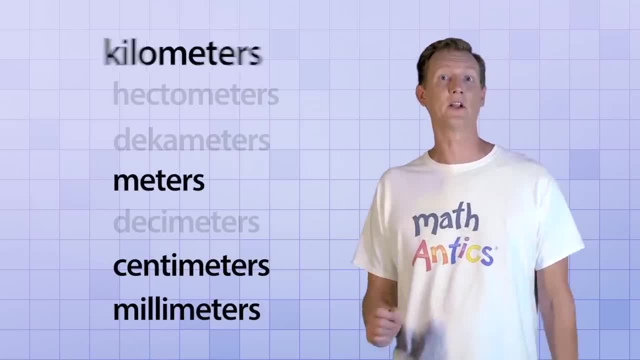 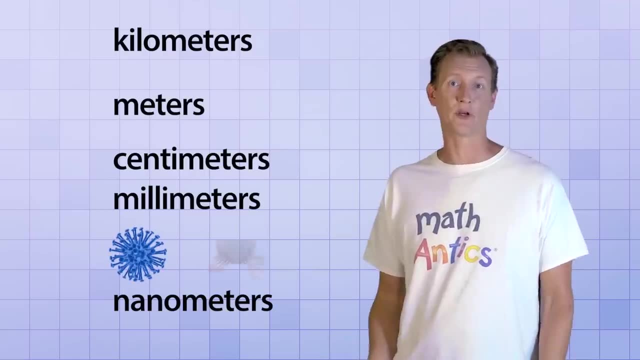 And they are the millimeter, the centimeter, the meter and the kilometer. Oh, and, of course, nanometers are commonly used when referring to teeny tiny stuff like microbes or computer chips. A nanometer is 1, one billionth of a meter. 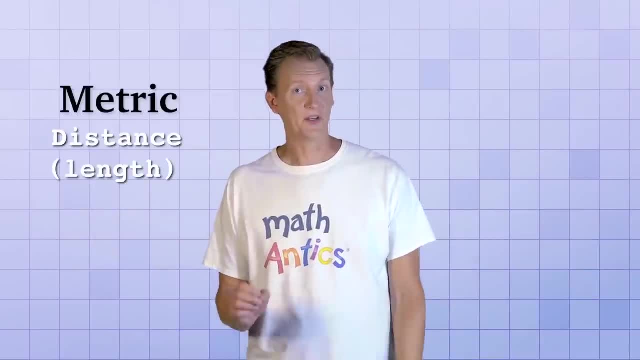 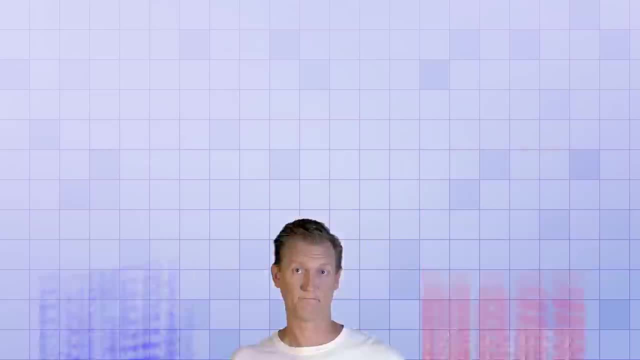 So that's how metric units of distance or length work. But there's another important quantity that uses the same powers of physics: It's the number of nanometers, It's called the 10 prefix pattern, and that's mass or weight. 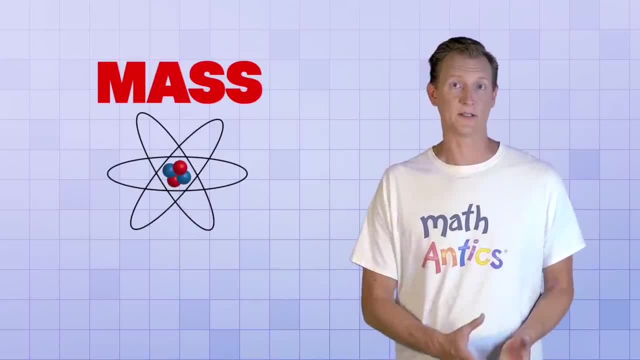 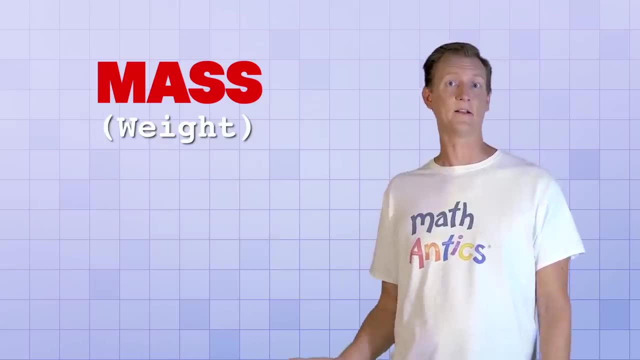 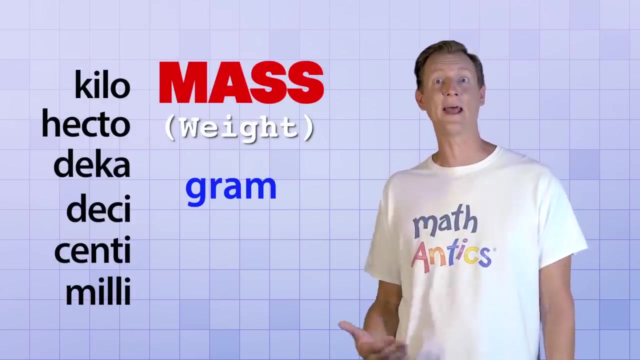 Mass is a measure of how much actual matter an object contains which is closely related to its weight on Earth. In the metric system, the basic unit of mass or weight is technically the kilogram, But we're going to start with just the plain old gram, to see how the same prefix pattern we used for length can be used for mass also. 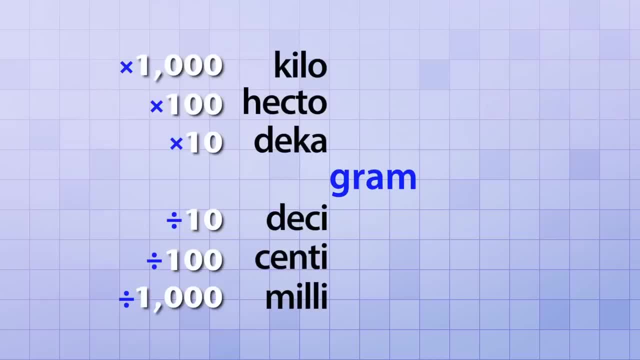 For reference, a gram is the amount of mass equivalent to 1 cubic centimeter of water. A decagram is 10 times bigger than a gram. A hectogram is 100 times bigger And a kilogram is 1000 times bigger. 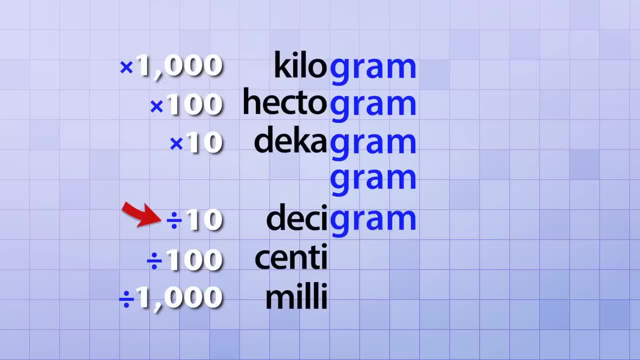 And similarly, a decagram is 10 times smaller, or one tenth of a gram, A centigram is 100 times smaller, or one hundredth of a gram, And a milligram is 1000 times smaller, or one thousandth of a gram. 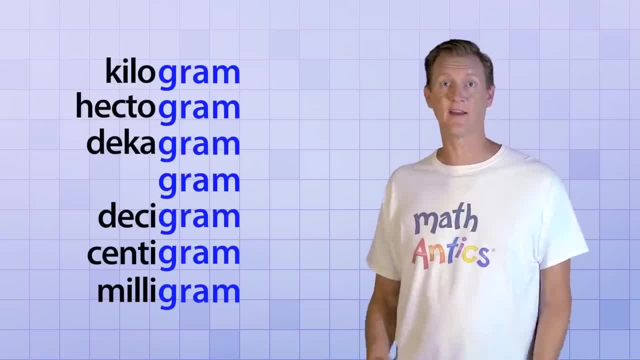 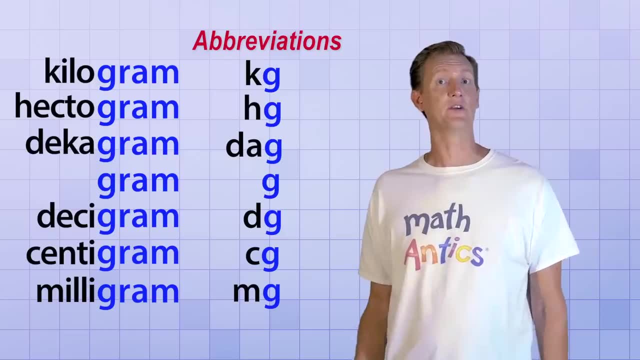 See, the same pattern is used And all of these units of mass have abbreviations. also. The pattern of abbreviation is similar to the metric units of length- length- but instead of an M for meters, you use a G for grams. KG is kilograms, MG is milligrams, and so on. 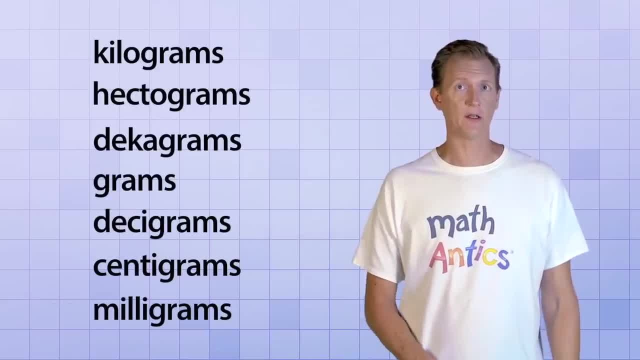 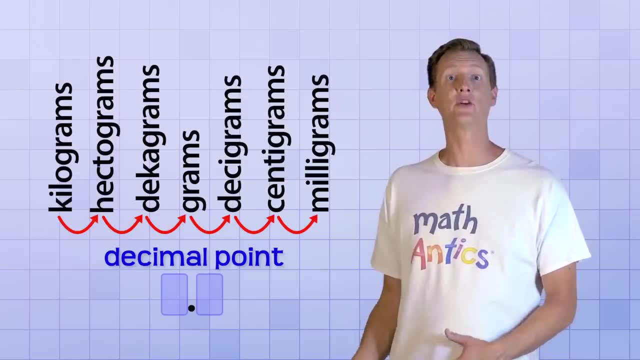 Again, because these units of mass are based on powers of 10, you can convert between them just by shifting the decimal point. You can convert to the next smaller metric unit by shifting the decimal point to the right, which is equivalent to multiplying by 10.. 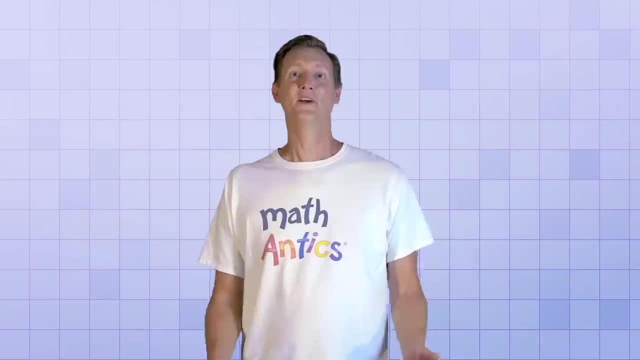 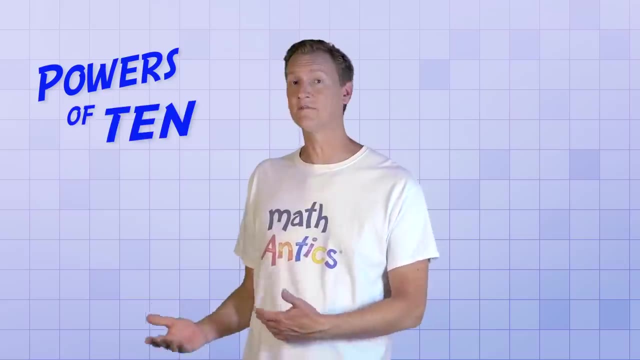 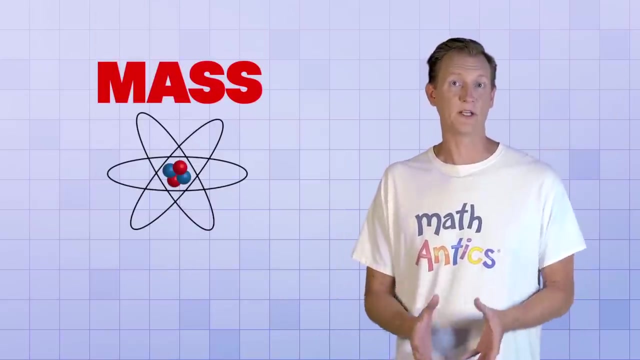 A nanometer is 1 one-billionth of a meter, So that's how metric units of distance or length work. But there's another important quantity that uses this same powers-of-10 prefix pattern, And that's mass, or weight. Mass is a measure of how much actual matter an object contains, which is closely related to its weight on Earth. 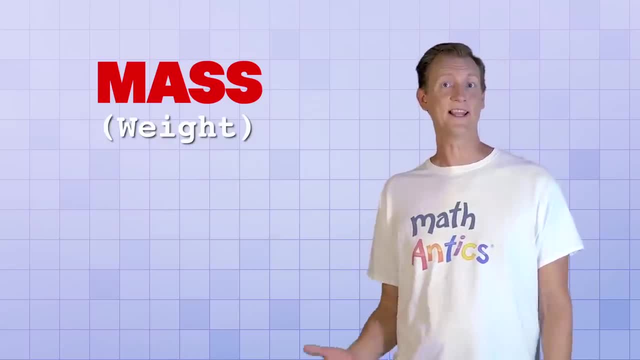 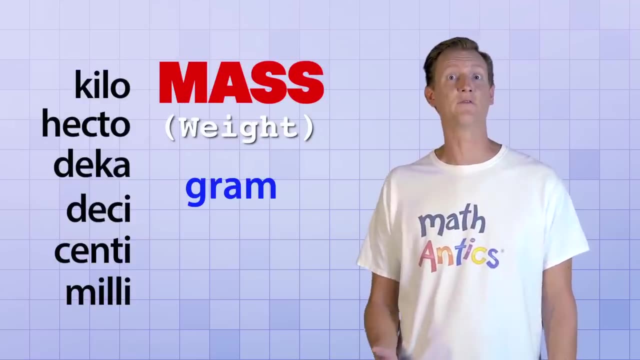 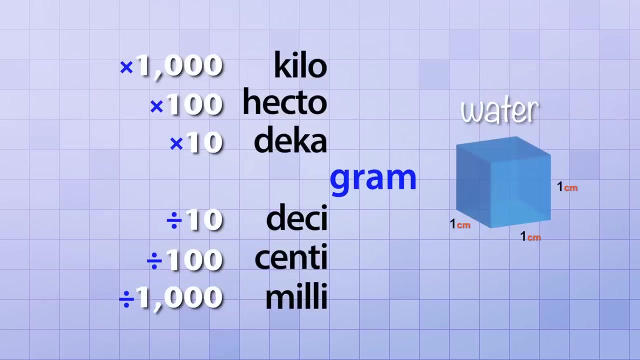 In the metric system, the basic unit of mass or weight is technically the kilogram, But we're going to start with just the plain old gram to see how the same prefix pattern we used for length can be used for mass also. For reference, a gram is the amount of mass equivalent to 1 cubic centimeter of water. 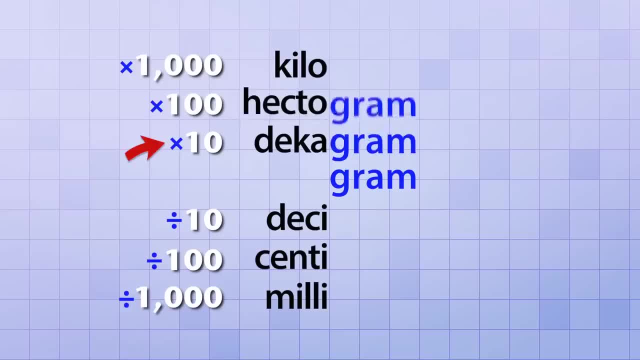 A decagram is 10 times bigger than a gram, A hectogram is 100 times bigger and a kilogram is 1,000 times bigger, And similarly, a decigram is 10 times smaller, or 1 tenth of a gram. 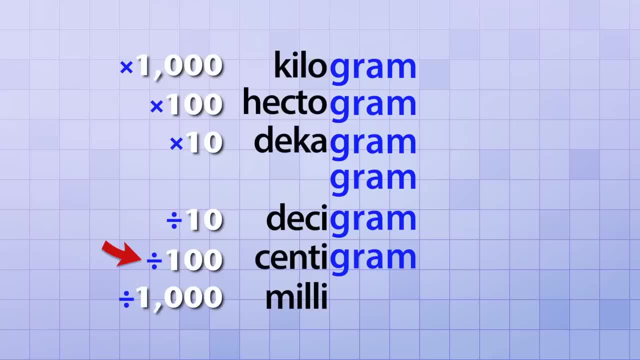 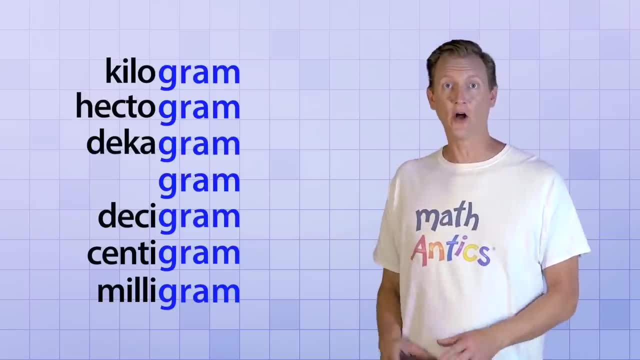 A centigram is 100 times smaller, or 1 hundredth of a gram, And a milligram is 1,000 times smaller, or 1 thousandth of a gram. See, The same pattern is used And all of these units of mass have abbreviations also. 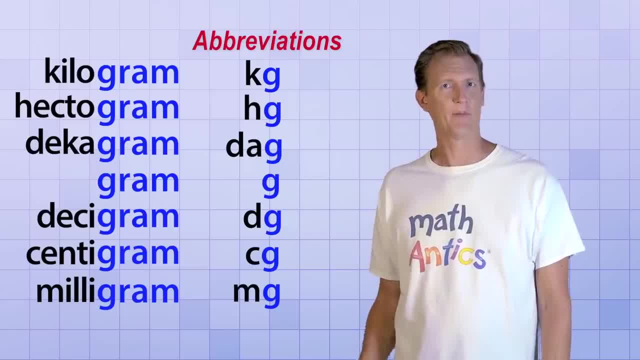 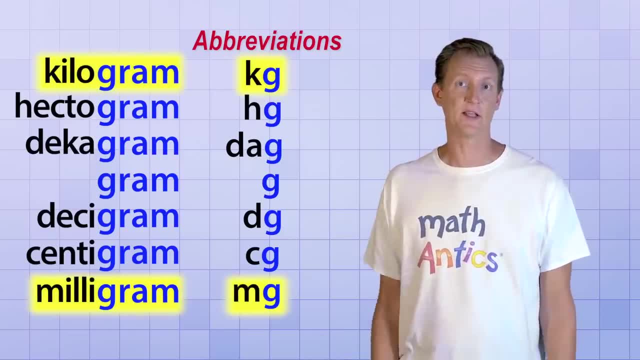 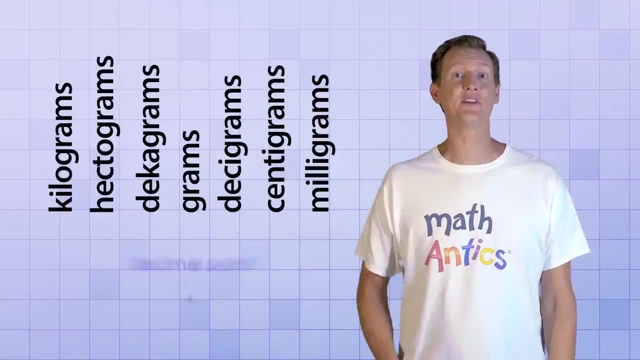 The pattern of abbreviation is similar to the metric units of length, But instead of an M for meters, you use a G for meters, G for grams, KG is kilograms, MG is milligrams, and so on. Again, because these units of mass are based on powers of 10, you can convert between them just by shifting the decimal point. 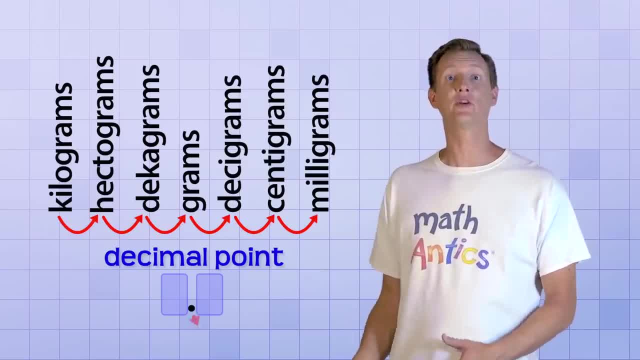 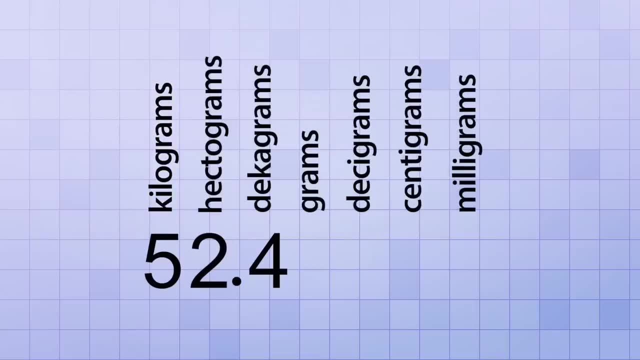 You can convert to the next smaller metric unit by shifting the decimal point to the right, which is equivalent to multiplying by 10.. 5.24 kilograms is the same as 52.4 hectograms, which is the same as 524 decagrams. 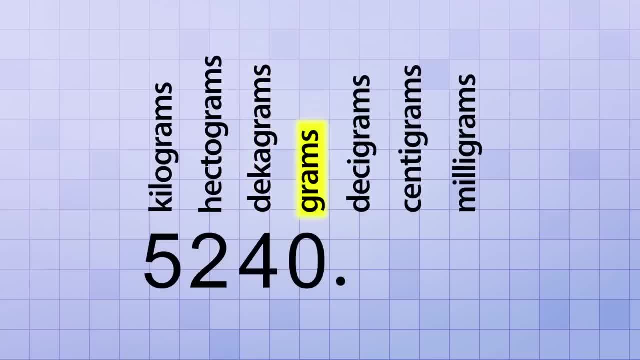 which is the same as 5,000 kilograms, And so on. And you can convert the next bigger metric unit by shifting the decimal point to the left, which is equivalent to dividing by 10.. 16.3 milligrams is the same as 1.63 centigrams, which is the same as 0.163 decigrams, which is the same as 0.0163 grams, and so on. 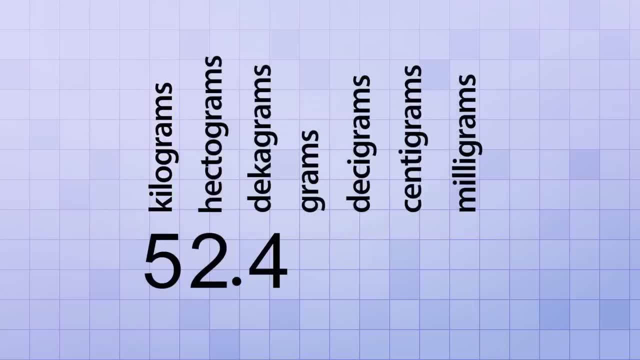 5.24 kg is the same as 52.4 ha, which is the same as 524 dg, which is the same as 5240 g, and so on, And you can convert to the next bigger metric unit by shifting the decimal point to the left, which is equivalent to dividing by 10.. 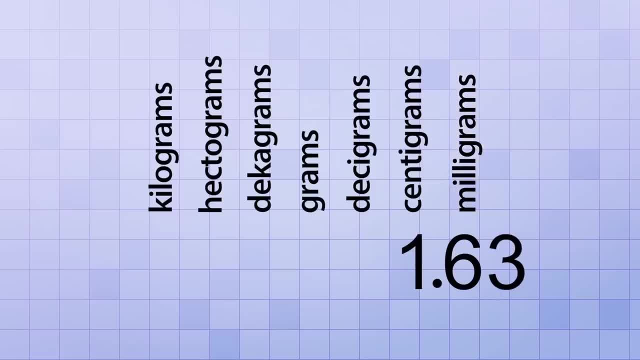 16.3 mg is the same as 1.63 cg, which is the same as 0.163 dg, which is the same as 1.163 dg, which is the same as 1.163 dg, which is the same as 10. mówią. 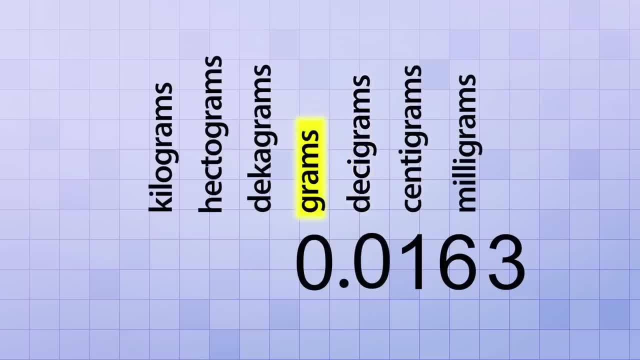 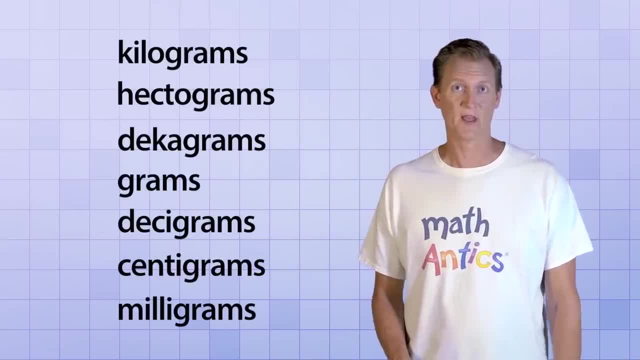 as 0.0163 grams and so on, But, as was the case with units of length, many of these units of mass are not used as often as the others. For example, centigrams aren't as popular because people will usually just say 10 milligrams. 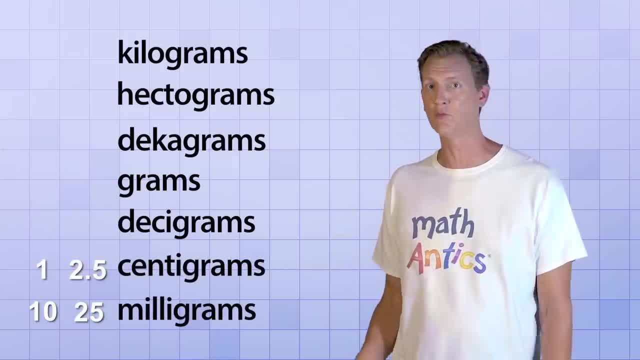 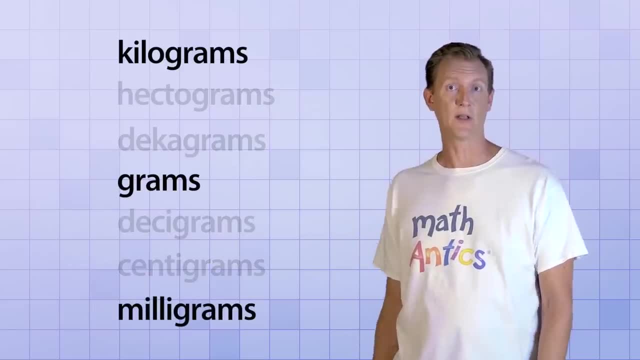 or 25 milligrams instead of 1 centigram or 2.5 centigrams. The units of mass that you'll most commonly encounter in everyday life are the milligram, the gram and the kilogram, so make sure you're familiar with those. 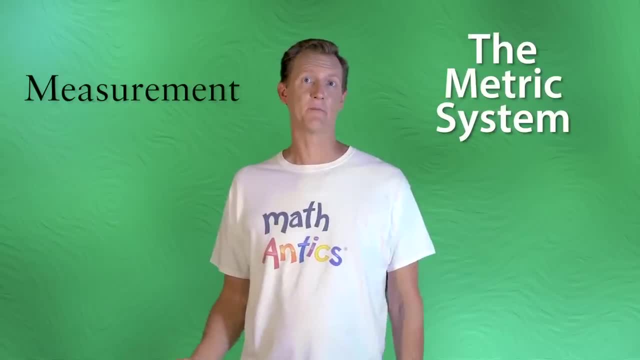 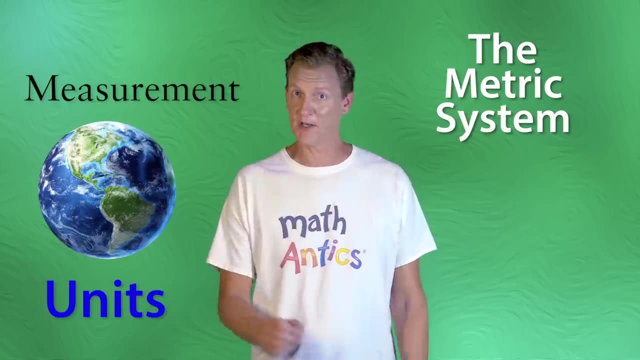 Alright, so that's the basic idea behind measurement and the metric system. Measurement helps us describe things in the world we live in and to compare them using units, And the units in the metric system are specially designed to play well with our base 10 number system. 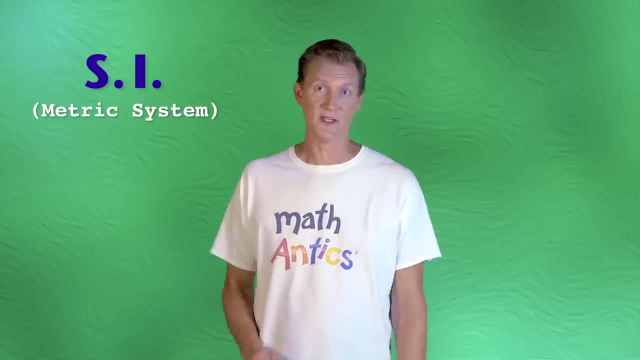 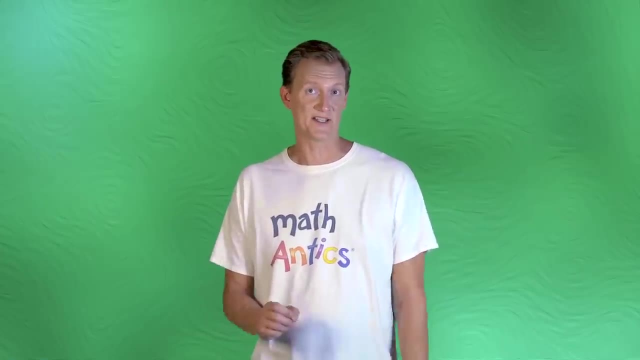 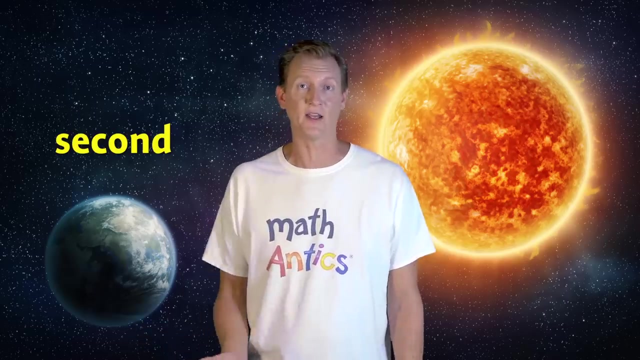 But it's important to know that the SI or metric system does use some units that are not based on powers of 10,, like time, for example. The basic SI unit of time is the second, But units of time that are larger than a second are still the traditional ones that are based on the motion of the Earth and the Sun. 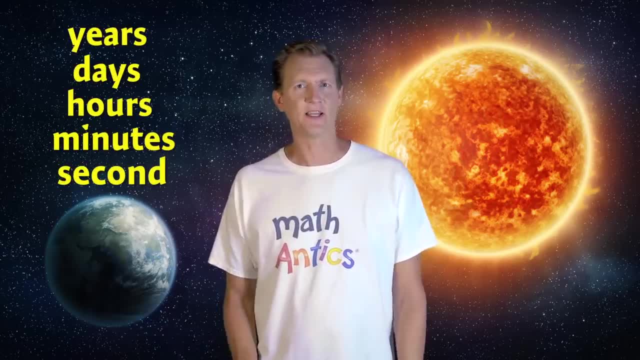 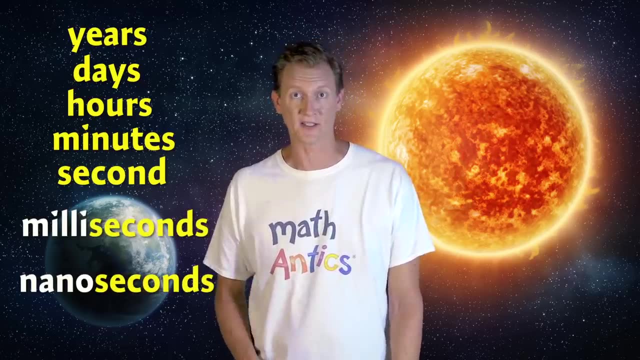 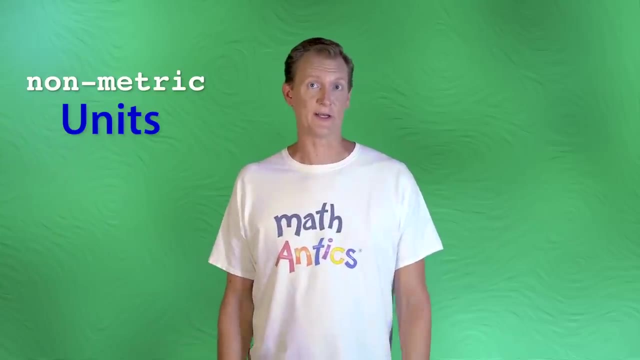 like minutes, hours, days and years. Fortunately, units of time that are smaller than a second do use the base 10 prefixes, such as milliseconds and nanoseconds. I wish I had more time to talk about time in this video and all the non-metric units that are still commonly used today, like feet or pounds. 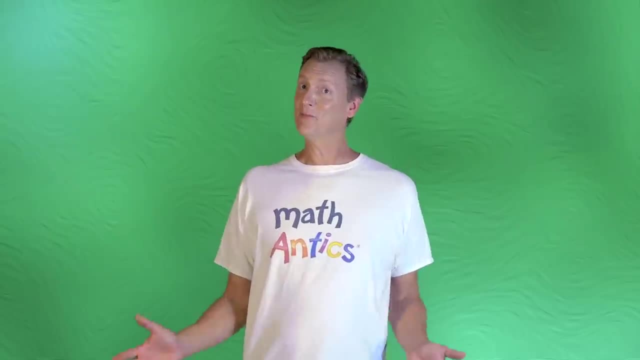